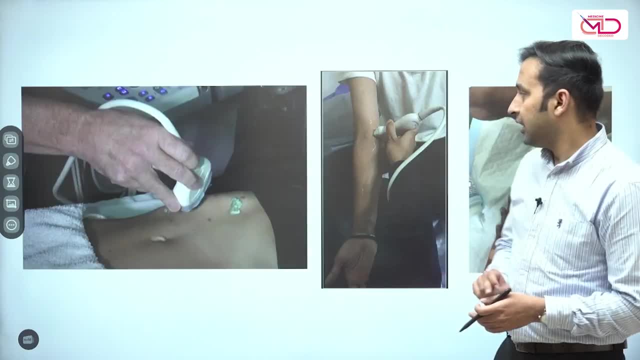 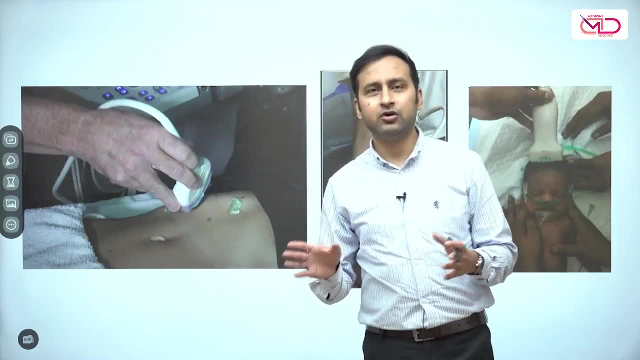 convenient and is a dynamic procedure. This is the common way in which ultrasound is done. This particular image shows you the transabdominal ultrasound. Most of you might have undergone some sort of sonography in your life, So what we do in a sonography is that, when the patient is lying down, 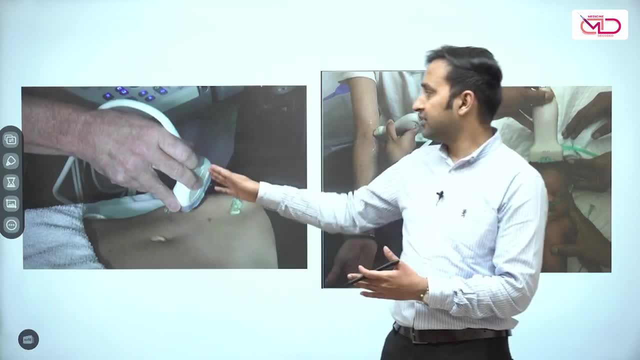 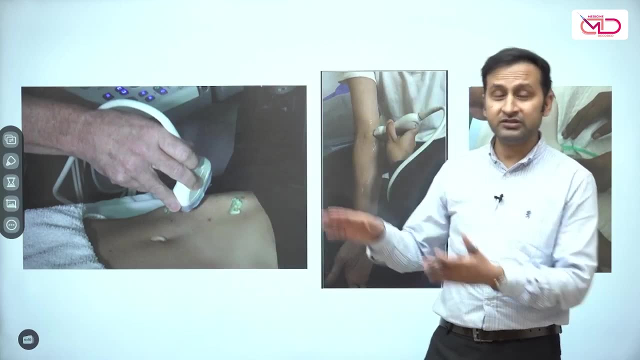 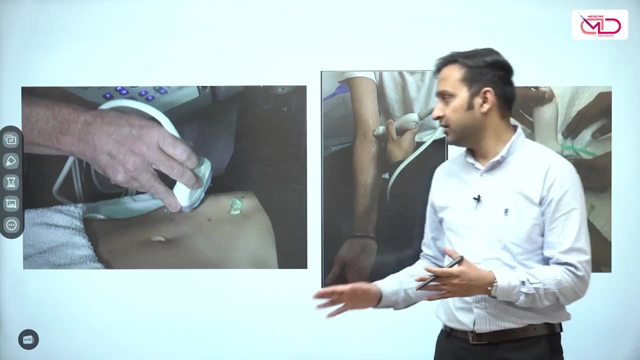 the doctor or the radiologist who's there. he places a probe, or a transducer, what we call it in our language, over the patient's body and there is a certain semi-solid substance which is placed over the patient's body because these sound waves cannot transmit through air. So we need certain, a certain thing which can act as a transmitting medium. 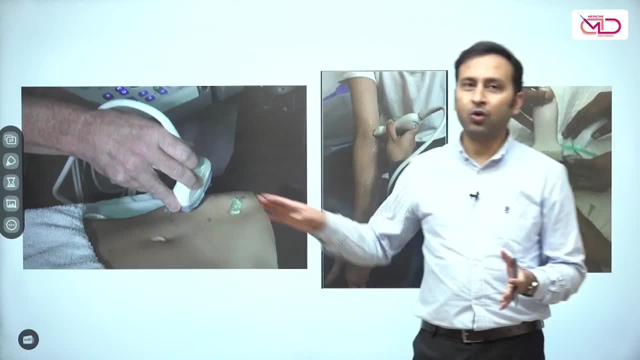 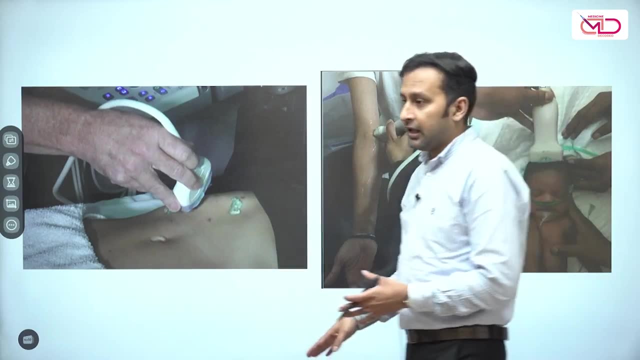 In our case, we use jelly. otherwise, you can use any liquid. even if you put water and you use the ultrasound probe over it, you can still have the same quality image while using this particular jelly. Now, why I put three images is that most of you might be knowing that ultrasound is used. 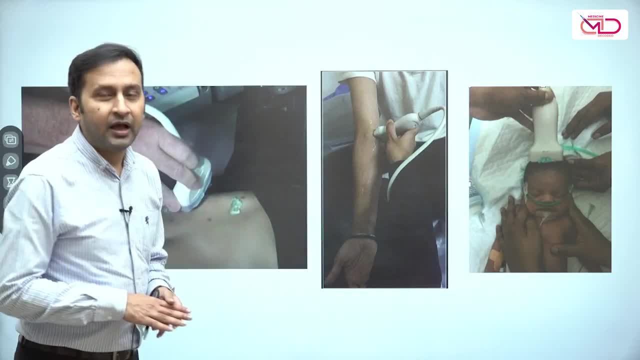 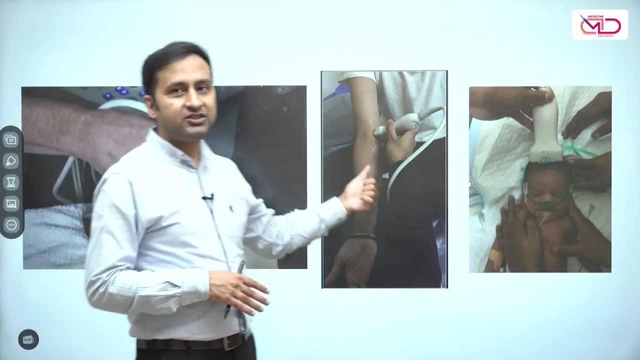 for abdomen and for pregnancies. but it is not true. Ideally, any soft tissue of the body can be imaged exquisitely well by using a normal sonography machine. In this particular image, ultrasound of the arm is being done, in which you can evaluate not only fluid containing structures. 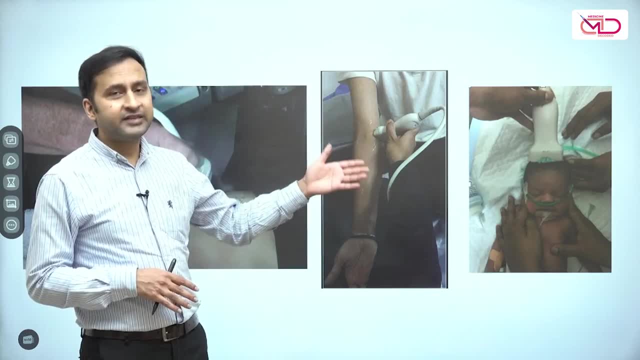 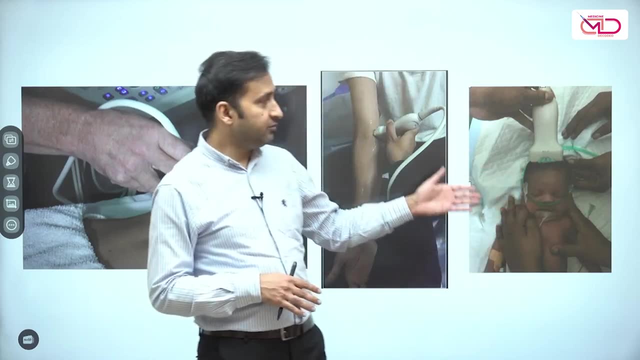 you can also see the soft tissues. you can also see nerves, muscles, everything. And you'll be surprised to know that in neonates, ultrasound can be used to see even the brain. Why ultrasound can be used in neonates and brain and not in adults. we'll be discussing about that in a subsequent 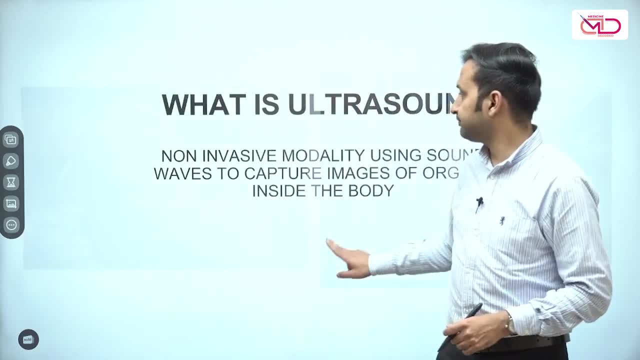 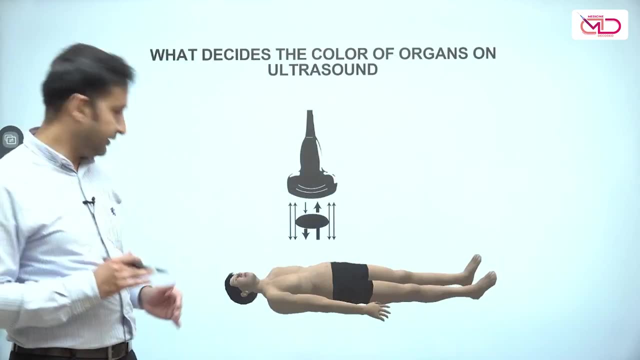 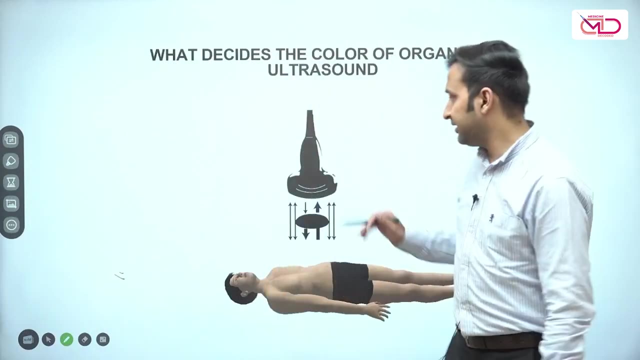 lectures in a subsequent section. So last time we've discussed about how does an image form in a x-ray. Now that was a bit different when we talk about ultrasound. the ultrasound image is formed by one single element, which is called as the transducer, or 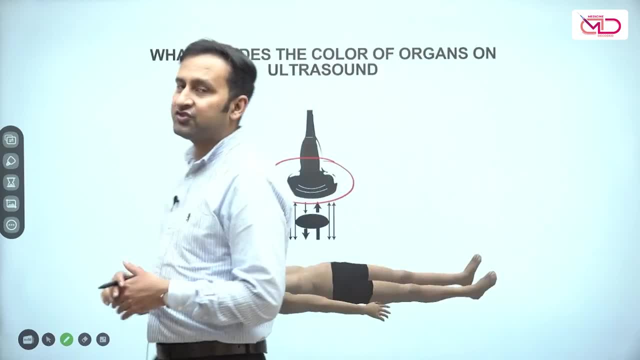 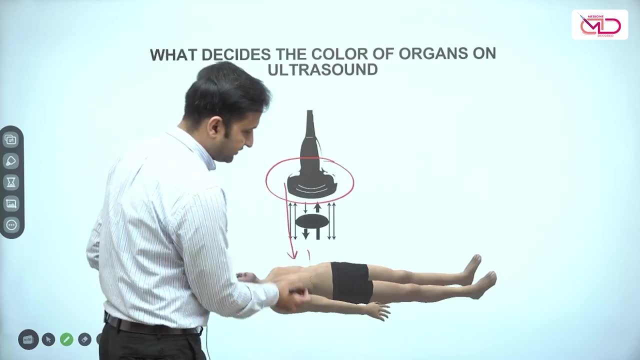 the probe. Now, what does the probe do? The probe is responsible for emitting the sound waves. Now, when the sound waves are emitted, a bit of the sound waves touch the patient. some of them are transmitted back. it's not transmitted after the beyond the patient and the others are reflected. 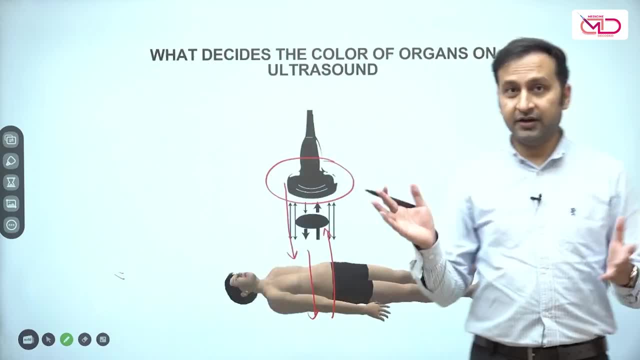 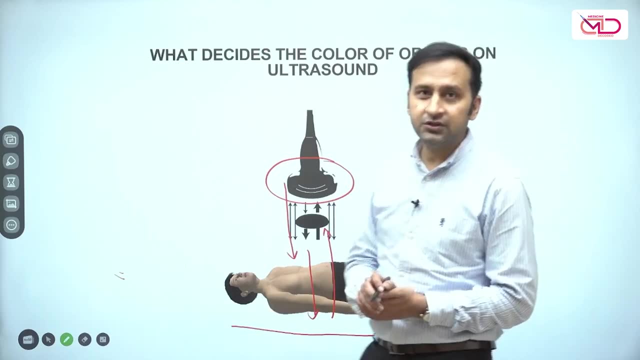 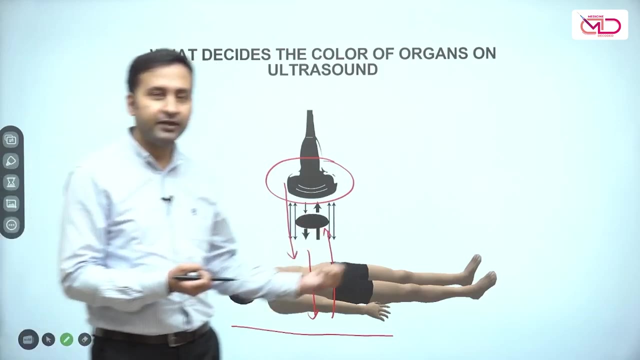 back Now. let's revise what we studied in x-rays. X-rays also, the same thing was happening, but there was a film which was placed just underneath the patient, which was responsible for what you call as receiving the images, receiving the x-rays which were transmitted through the patient's body. 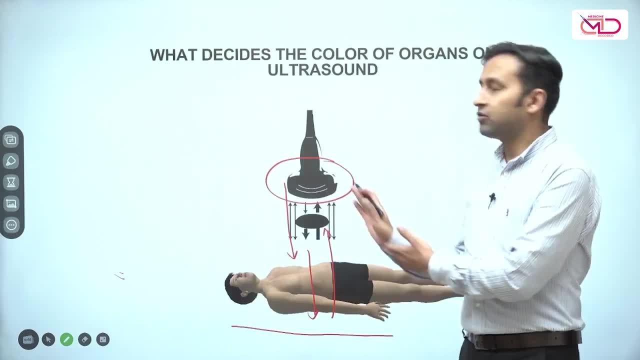 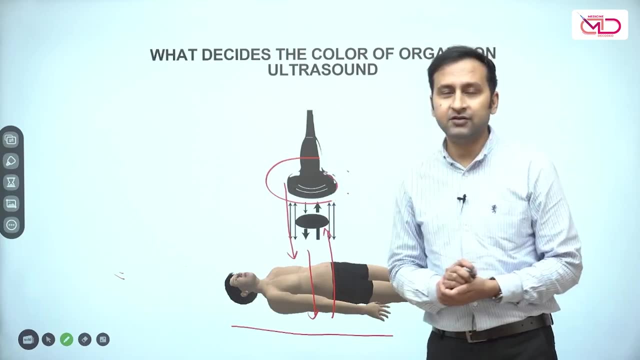 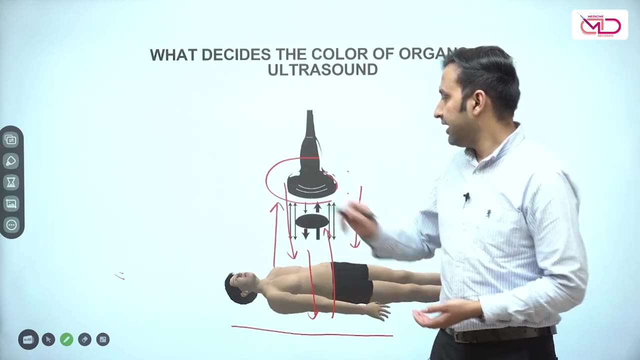 and the image was formed, But this is in complete contradiction to what we see in x-rays In this particular case. this transducer is a fascinating structure. it's a wonderful structure. not only is it responsible for emitting the sound waves, it is also responsible for accepting the received sound. 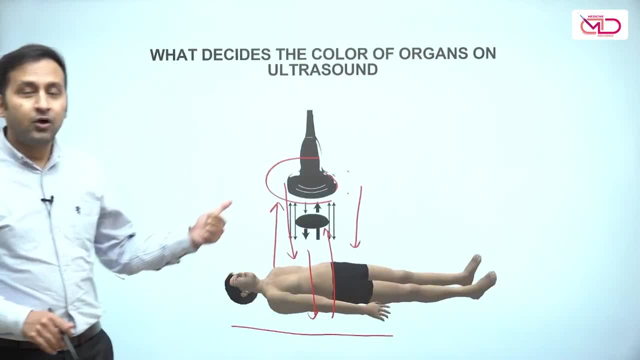 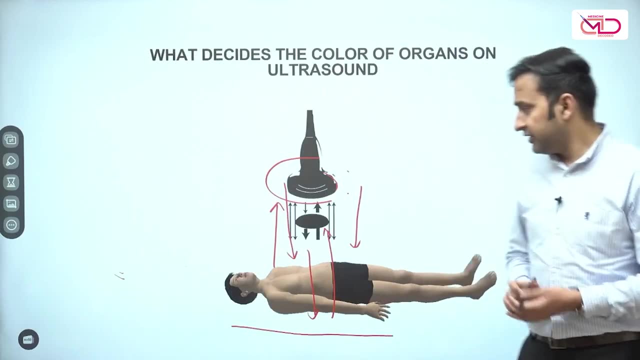 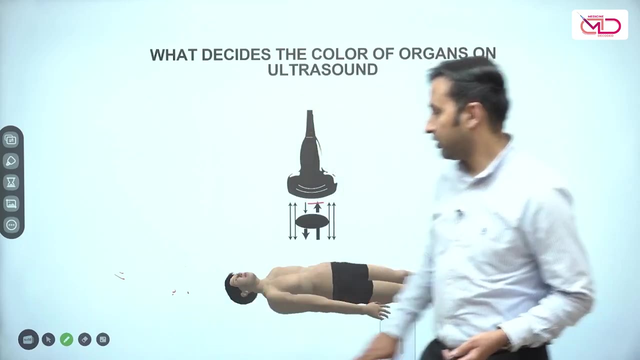 waves. So now what we can conclude? that only the image, the sound waves which are reflected back, will be taken up by the transducer and will form an image. So next question that might come to your mind is: when, when we're talking about sonography, is that what are the substances which are going to be transmitting the 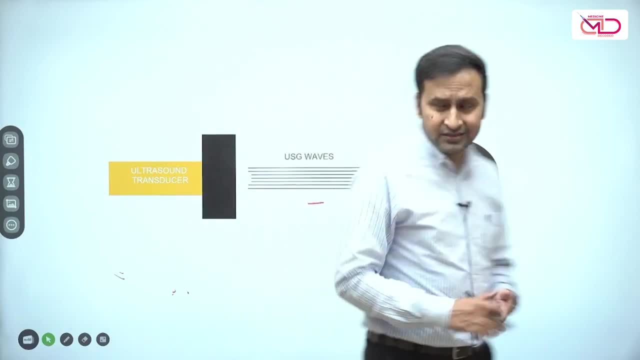 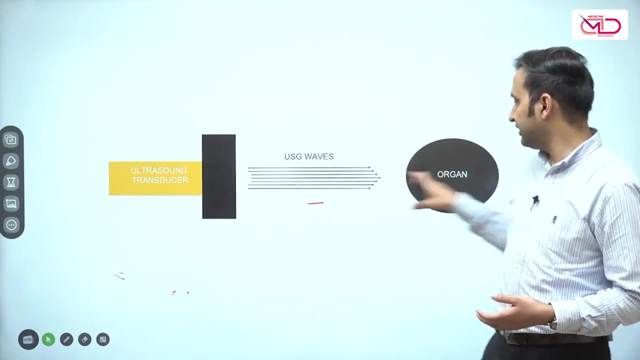 sound waves and what are the substances are going to be reflecting the sound waves? This is a schematic diagram. again, we can see that there is an ultrasound transducer which is generating the sound waves. this is that particular organ. the sound waves hit that organ. some are reflected. 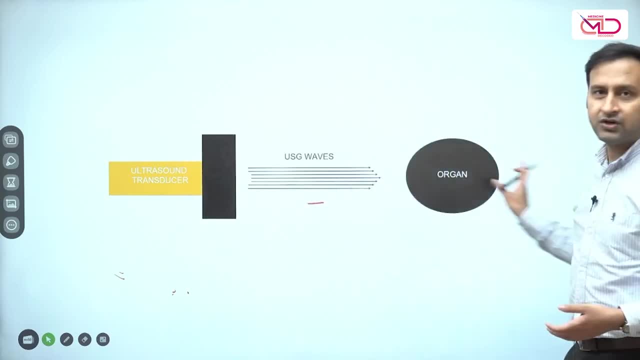 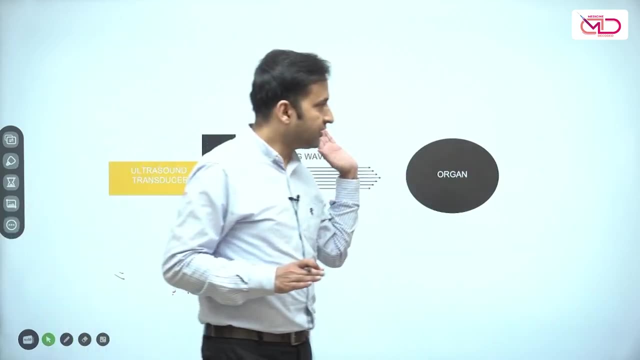 back which form an image on a transducer and whatever the sound waves are going to be passed off, they are going to be of no use to the ultrasound transducer because transducer won't pick them and all those sound waves which are transmitted will not produce any. 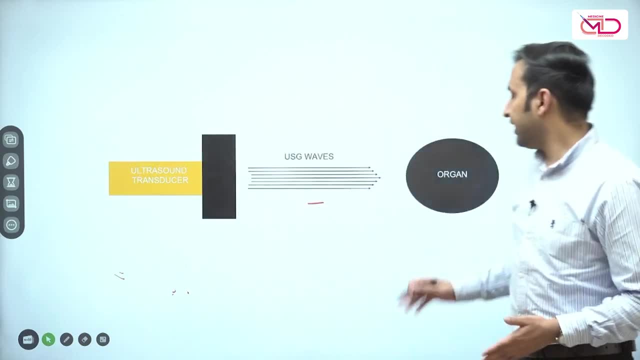 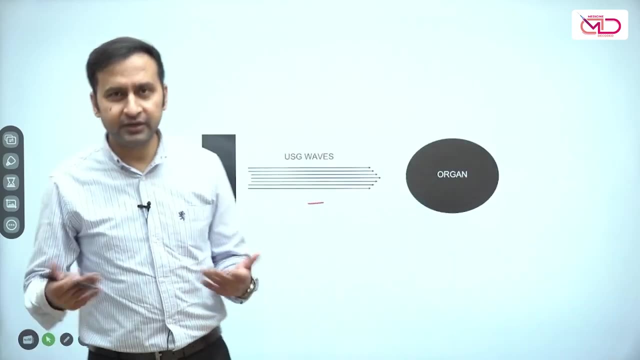 image on sonography and that will appear black. On the other hand, whatever images are going to be transmitted back to the ultrasound will produce some signal on the ultrasound machine. maybe it could. it could be white, it could be grey, it could be of some other shade. So, coming to the most basic, 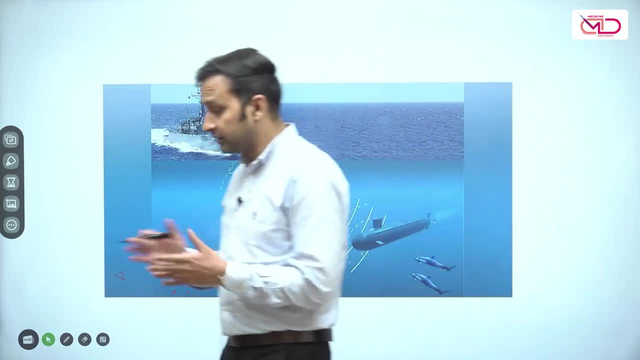 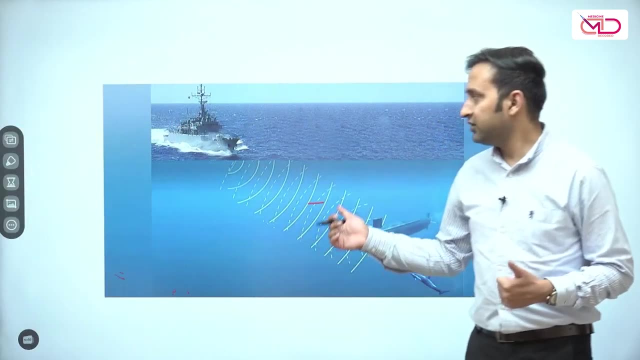 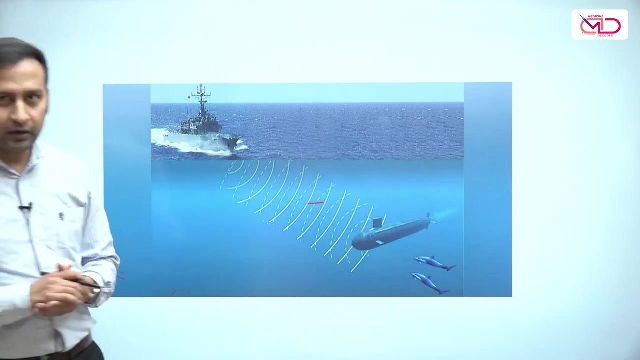 point: how does a particular object behave in front of ultrasound waves? To explain this, this is an example I've taken from the sonar. I hope that you- most of you- might be familiar with the sonar concept of sonar, that is, sound, navigation and ranging or radar. 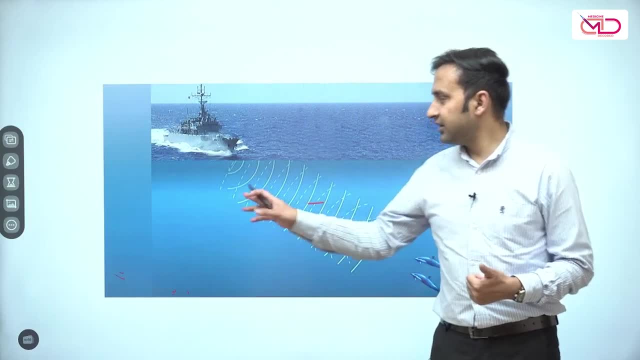 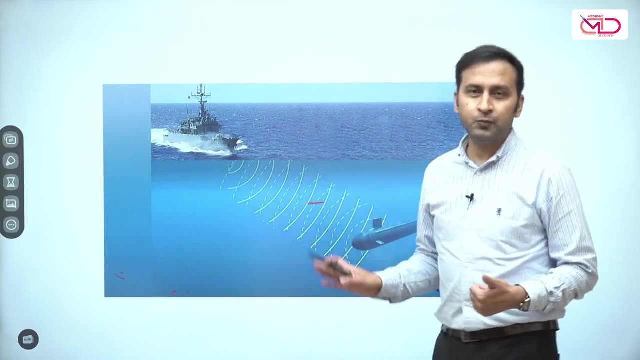 Now sonar waves like. what happens is that sonar is the behaves very similar to the ultrasound waves. in which what do these navy machines and these submarines do? they emit sound waves. they are very similar to the ultrasound waves. and once these sound waves 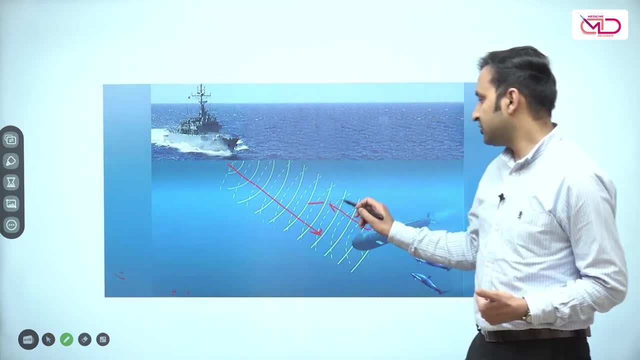 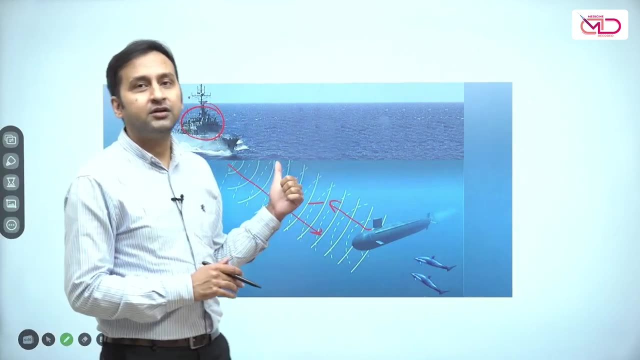 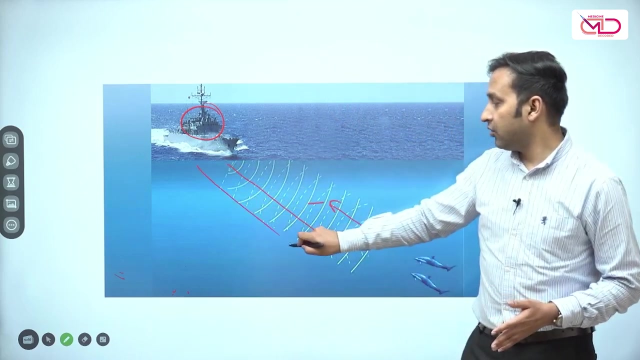 are transmitted. a bit of these sound waves are reflected in solid submarines and whatever they are reflected, they are picked up by the transmitter. here This is very similar to the transducer of the ultrasound that we see. That means when we are using an ultrasound machine, whatever the sound waves or the ultrasound, 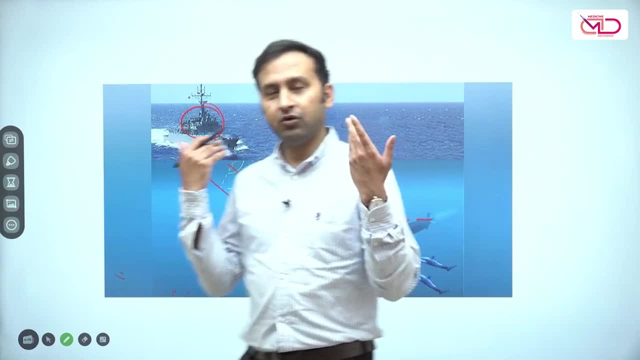 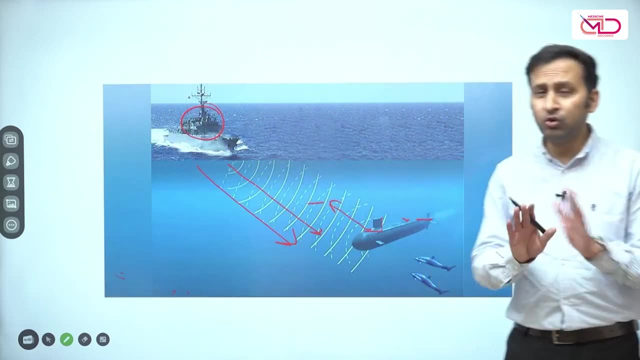 waves are going to pass through liquid. they are going to behave freely. they are never going to return because liquids are not going to produce any deceleration to the movement of sound. they are going to produce no restriction to the movement of sound. 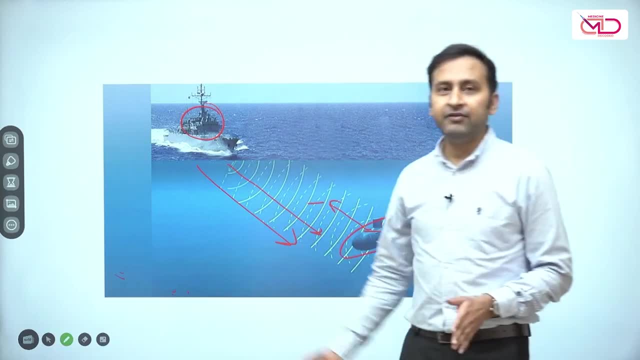 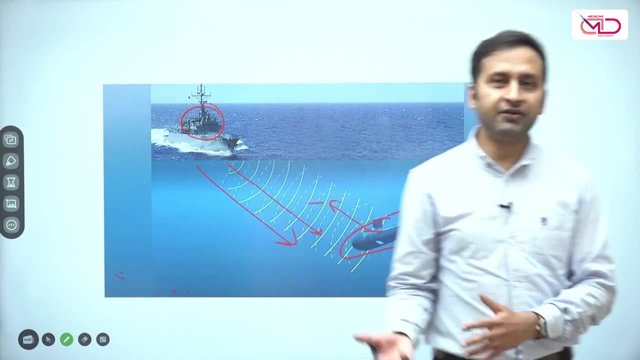 On the other hand, any solid substance, depending upon the density, will reflect major power part of the sound waves and whatever is reflected back, obviously it is going to produce some color. The more the sound waves are reflected, the brighter the image is going to be appearing. 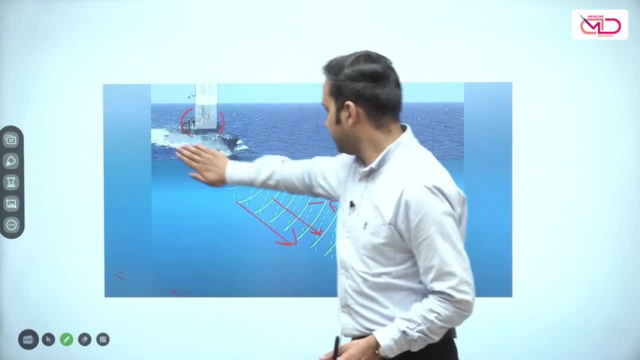 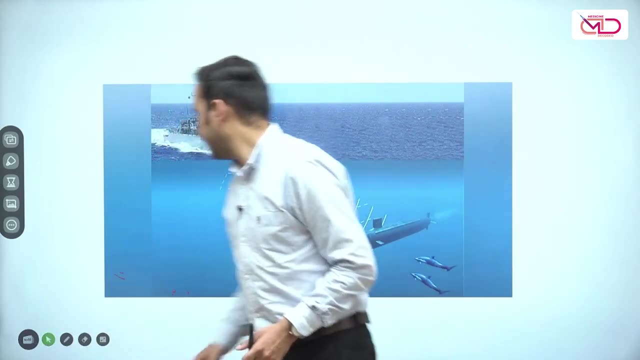 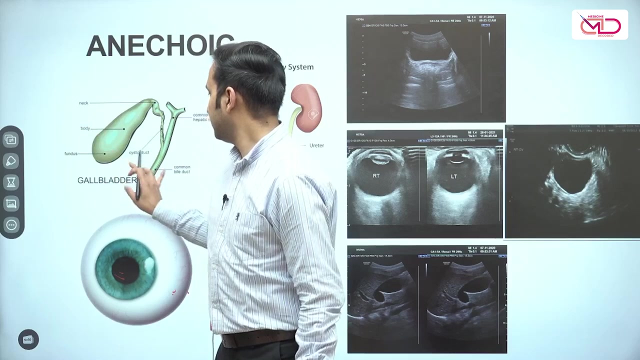 on the ultrasound. So this was all about the basic mechanism of sonography. Now coming on to the common objects that we see in our day to day life, on sonography, But before that I would just like to stress the terminology: An echo means echo, echo means echo. 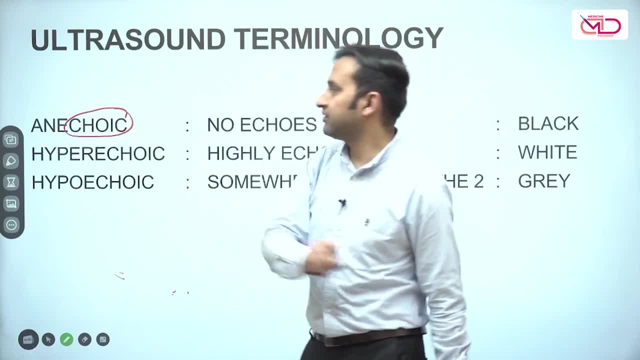 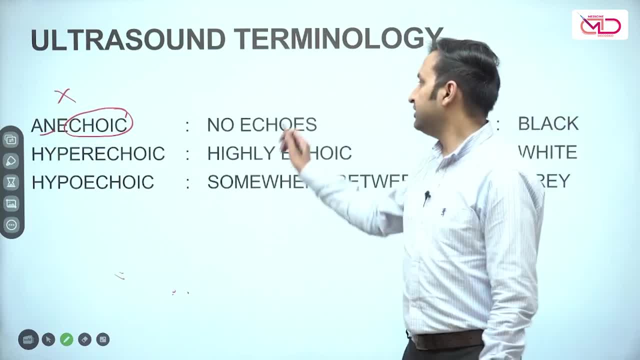 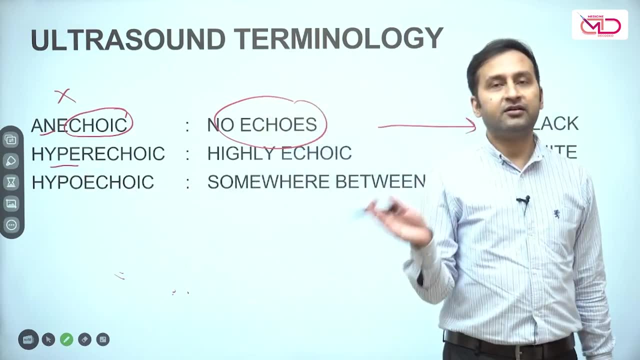 to be no echoes which are going to be reflected back. the image that is going to be formed will be completely black. A substance which is hyperechoic means it is going to retransmit. it is not going to transmit any sound waves. it is going to reflect majority of the sound waves and, as a result, 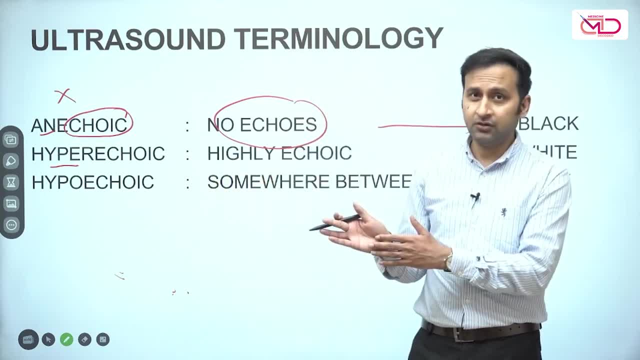 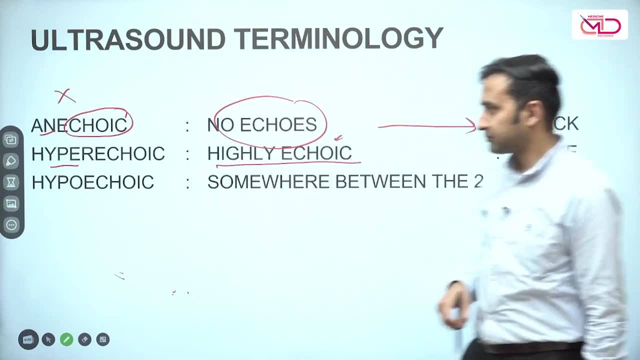 a large number of sound waves are going to be reduced by the transmitter or the transducer and, as a result, this will be highly echoic and this will appear completely white. Hypoechoic is a related term. it is somewhere between hyperechogenic and completely anechoic. 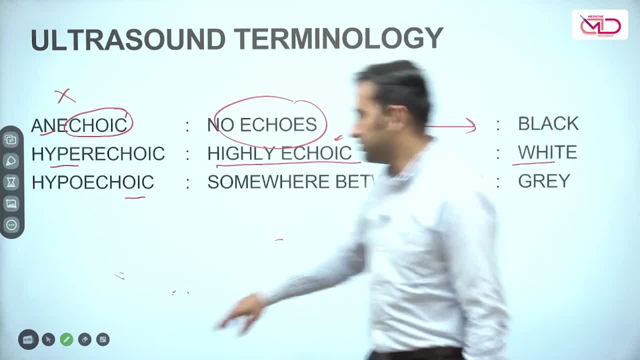 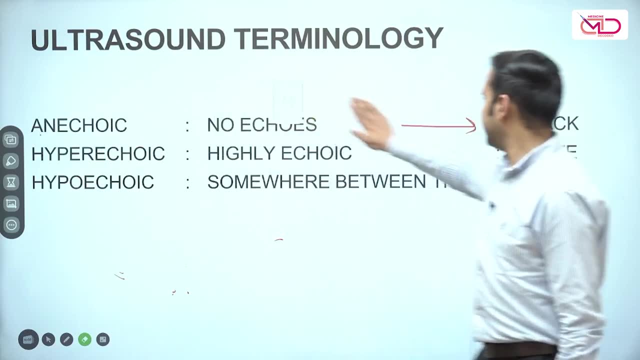 it could be in varying shades of grey, but it is relative. A substance is going to be hypoechoic in respect to another structure. So, with these words, let us see the common things that we see in our day-to-day life. on sonography: 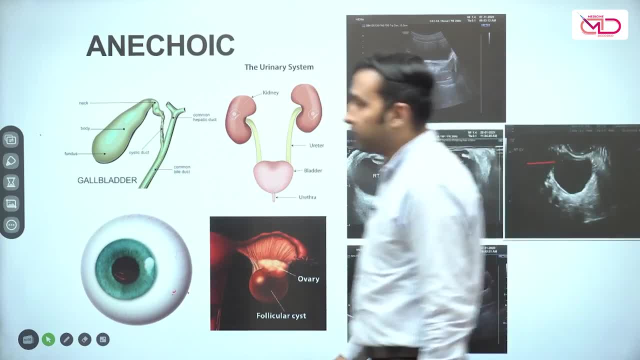 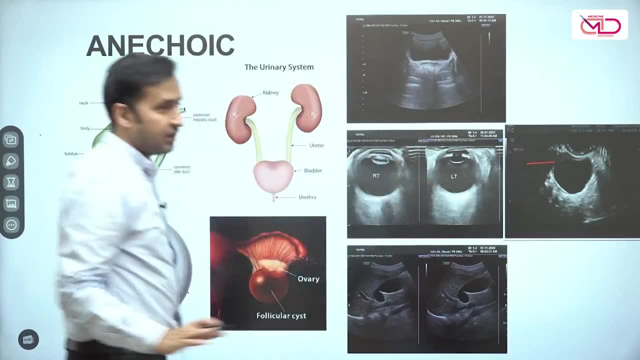 Now, starting off with this particular image. first, What we can see in this particular image. we can see that there is a substance which is present, which is giving us a black colour. Before I go ahead, I will tell you one more thing. one more funda of ultrasound is that 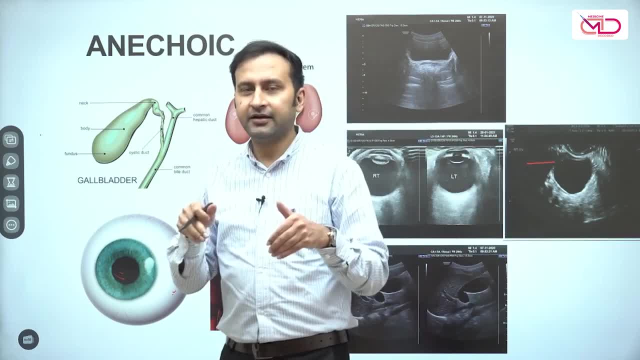 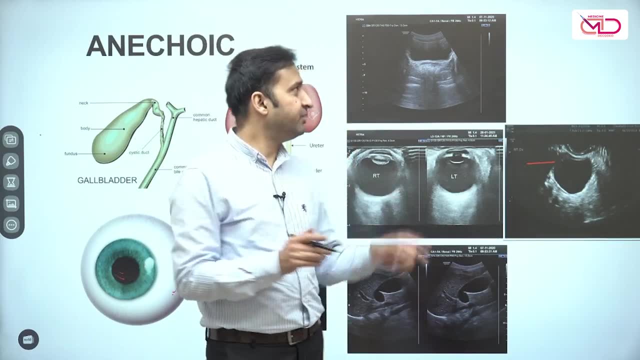 the ultrasound beams. they travel in just like in parallel direction, like X-rays or any other rays. So the thing that is going to strike the ultrasound beam first is going to be appearing closest to the screen In this particular case. what I want to say is that 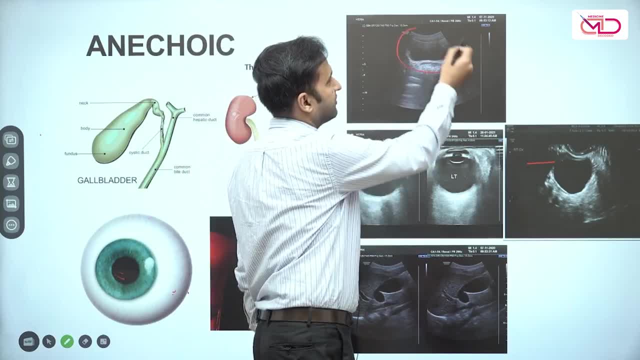 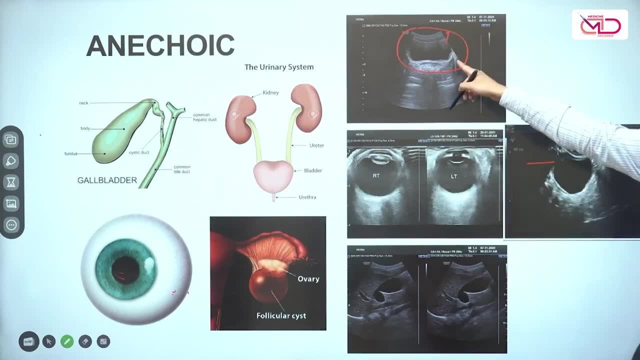 If, If this substance is closest to the screen surface, it means it is closest to the ultrasound probe. Now let us look at this particular structure which we can see. it is completely black. So black would mean anechoic, because it is not producing any echoes. 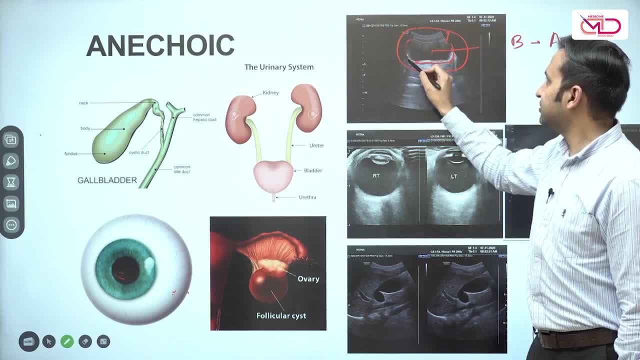 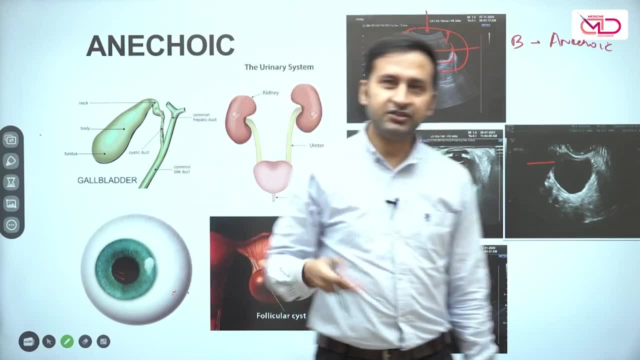 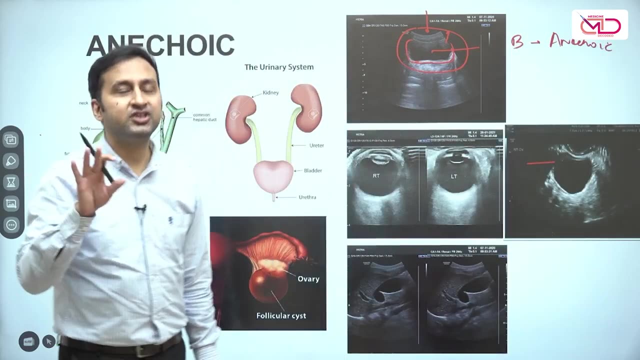 We can see that this structure has a ball, This structure has a quadrilateral shape and this structure is present just beneath the skin because the transducer is present just over the skin surface. If I tell you that, while I was imaging this organ, the transducer was placed just above. 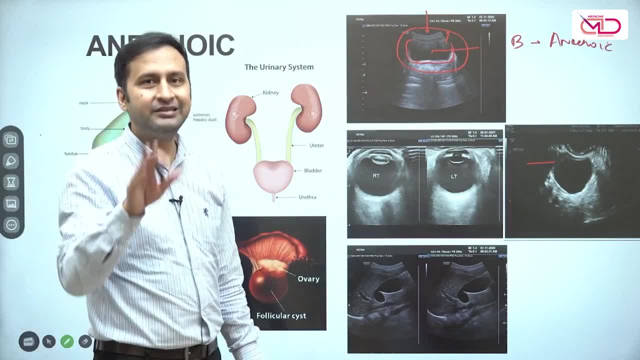 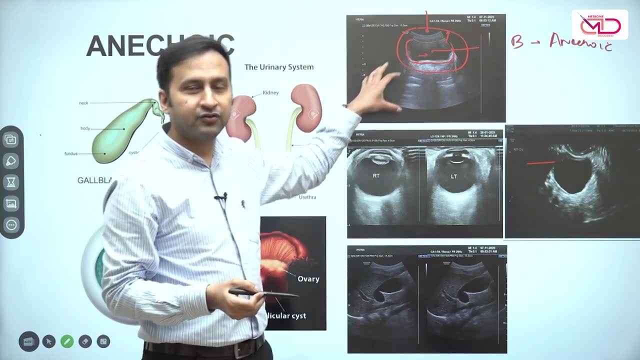 the pubic symphysis or the suprapubic region. you can easily reduce. This is a structure which is fluid filled, present in the suprapubic region, has a quadrilateral shape and is a wall of structure, So it is nothing but the urinary bladder. 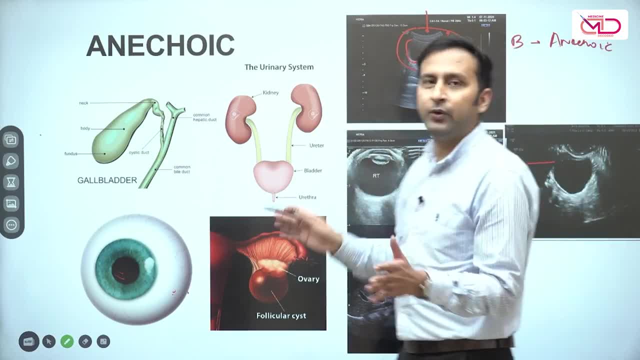 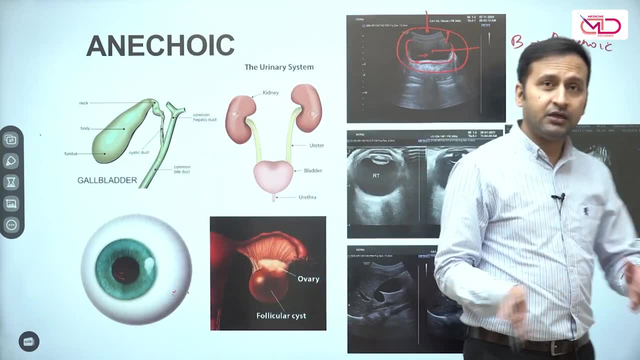 So, going on with that analogy, any bladder which is containing fluid will appear black, and there are only two bladders in the body: the urinary bladder, and the other one is the gallbladder. So, keeping that in mind, I will show you another structure. 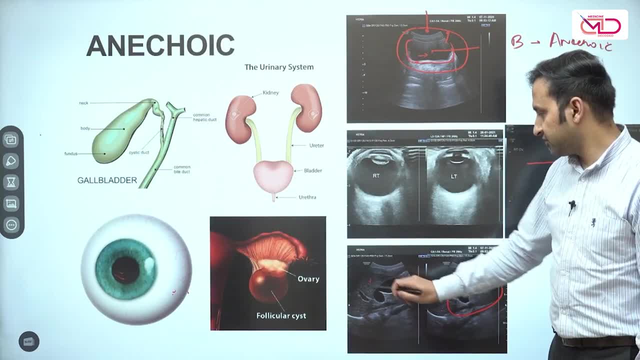 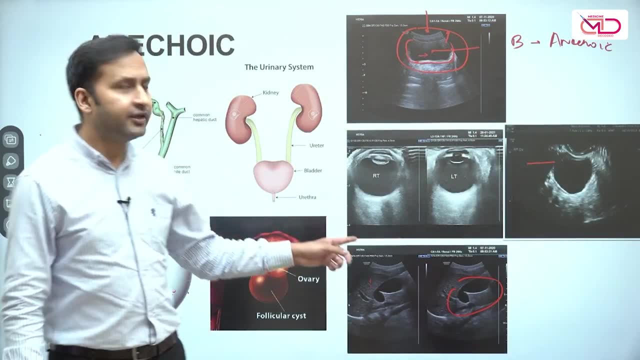 This is a pier-shaped structure. as you can see, I am not interested in this structure right now. Right now, I am interested in this particular structure, which is completely black. You can see that this black-colored structure has also got a thin wall, but it is not present. 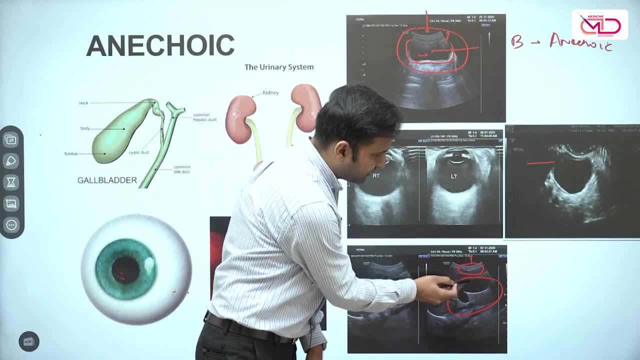 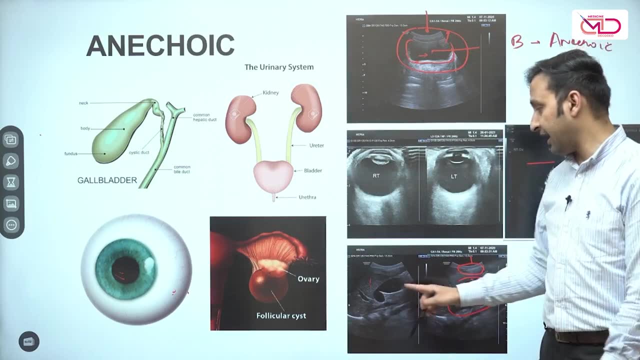 just beneath the skin You can see that there is a certain amount of tissue which is separating it from the skin surface. So we can deduce that this pier-shaped structure is a structure which contains fluid, because it is completely anechoic. It is black. 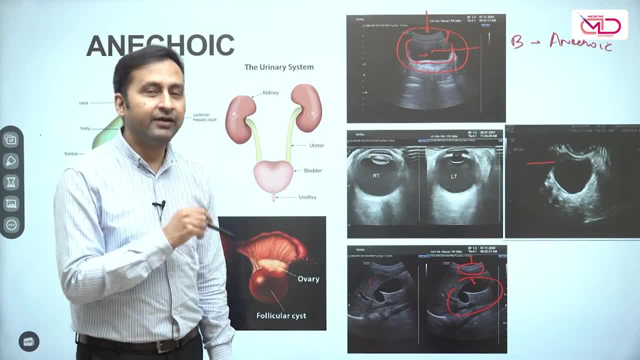 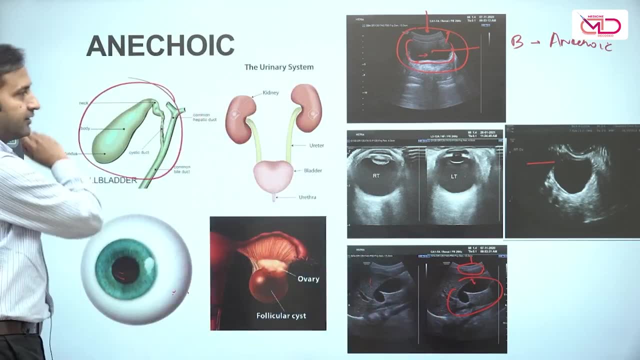 It is black from the skin surface. More importantly, if I tell you that I was imaging the right hypochondrium while I found the structure, then anybody of you can tell that this is nothing but the gallbladder. So we discussed about two bladders: the gallbladder and the urinary bladder. 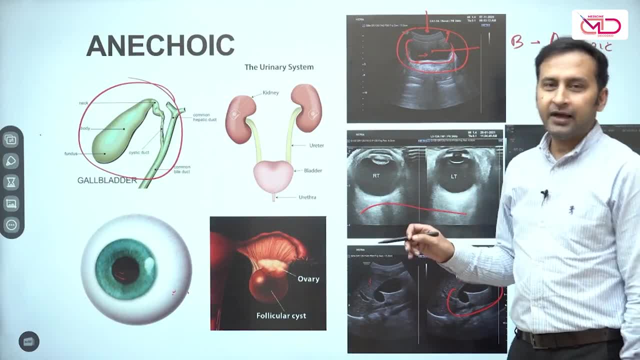 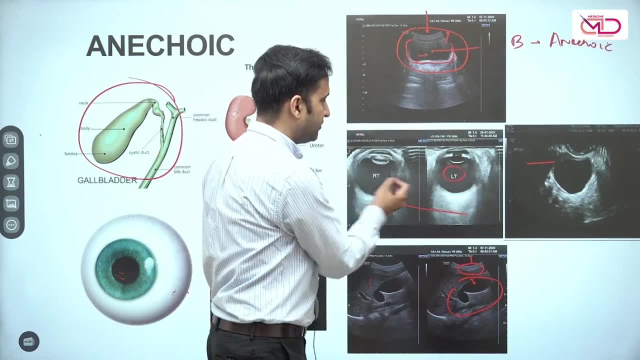 The third thing is these two paired structures, which are void structures. the majority of you can see by the shape that they look like human eye. indeed, they are the human eye. You can see that they are looking black because human eye is filled with vitreous humor which 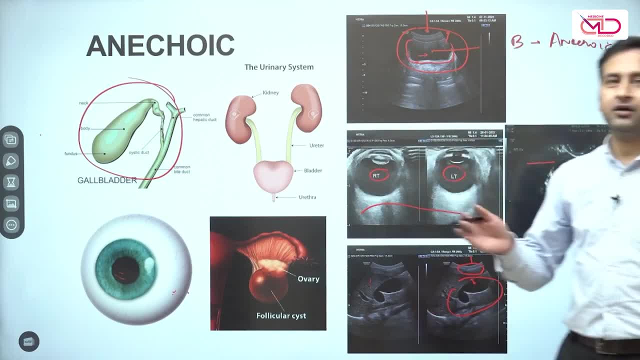 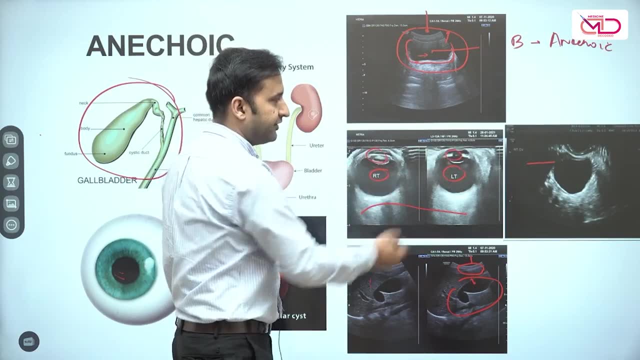 is again a fluid. It is not going to trans, It is not going to do what you call as reflect any sound waves and it is going to transmit all the sound waves. This you can also see that there is a certain amount of lens material which is present interiorly. 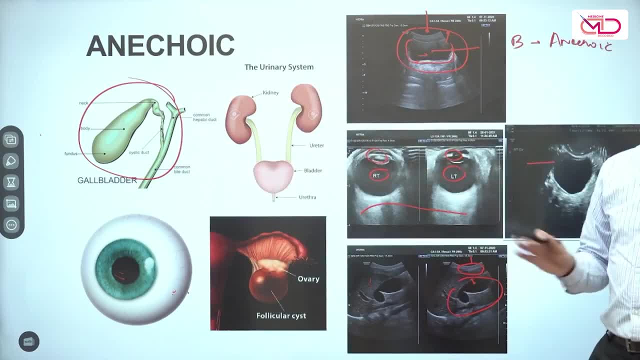 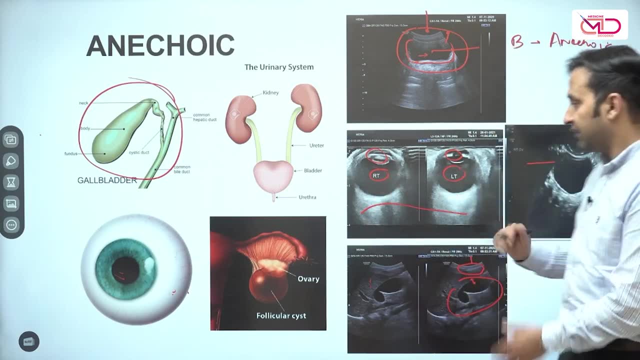 But the concept is anything which is transmitting almost all the sound waves to it will appear black: All these bladders, the eye, the UB and obviously the last thing which I left was the adenexal cyst. This is the adenexal cyst. 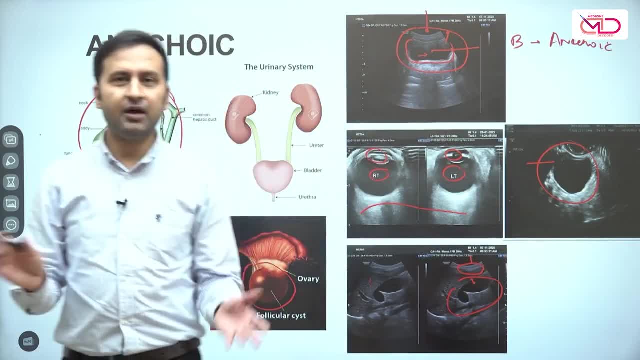 All the cysts, the simple cysts in the body, wherever they are present, whether they present in the kidney, whether they present in the liver, whatever they are present in the liver, whether they present in the ovary testes, anywhere, even in breast, they will be filled. 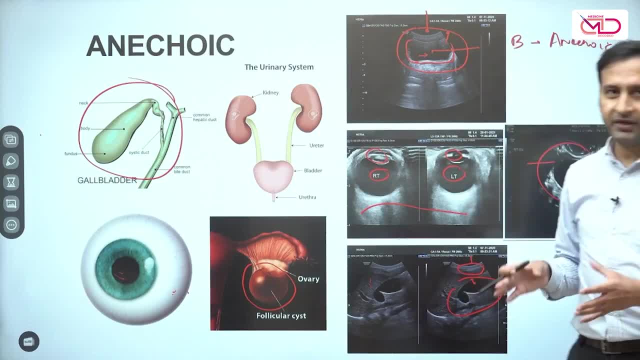 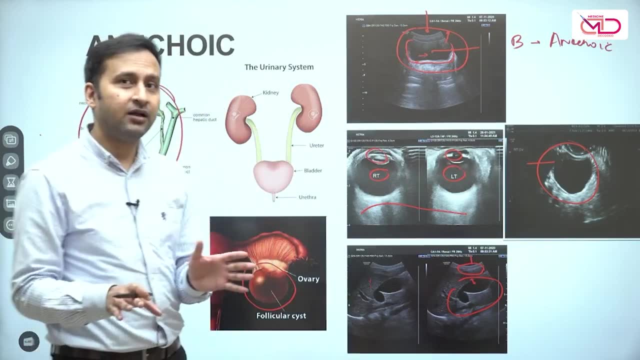 with fluid And until and unless they are complicated by some hemorrhage or something, because the fluid is completely anechoic, you will see them as very thin walled structures which have got no color. they will appear black or something which is anechoic. 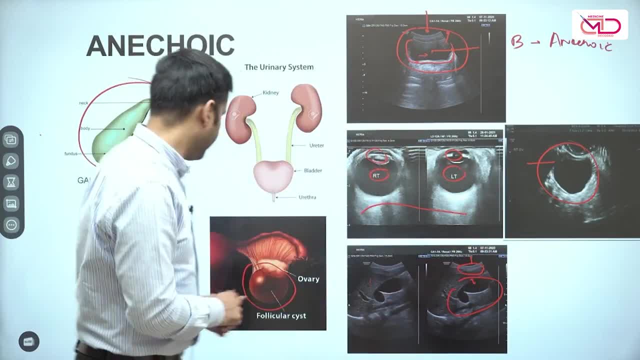 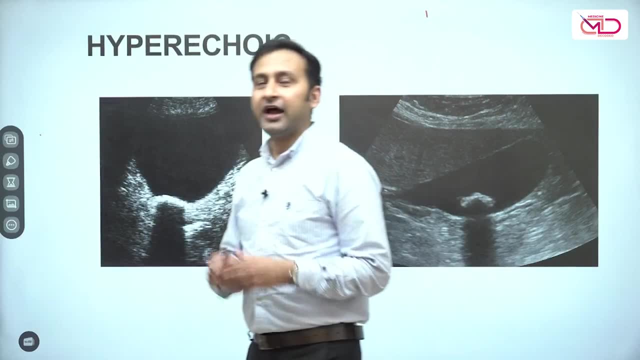 So this is how these anechoic structures look on sonography. Now moving ahead with the other spectrum. The other spectrum is that of hyperechoic substances. Now, hyperechoic substances, I told you, are those ones which are going to be. 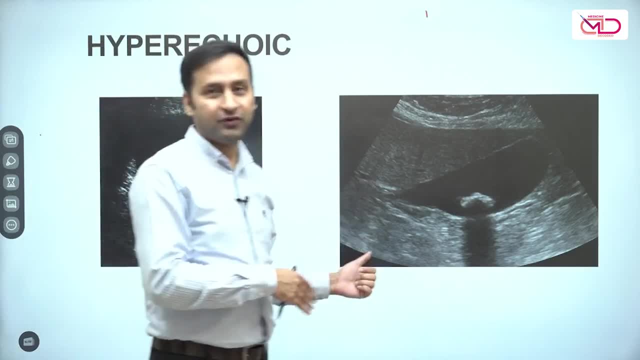 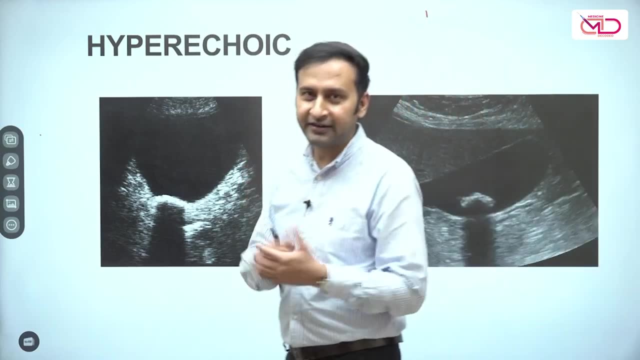 No, which are going to be reflecting majority of the sound waves. So those substances which are very hard will be reflecting majority of the sound waves. as we discussed, The higher the density, the more the sound waves are going to be reflected back. There are two major hard substances in our body, that is, the bone and the stone. 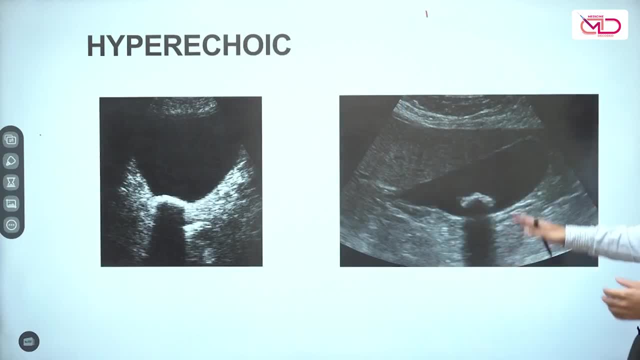 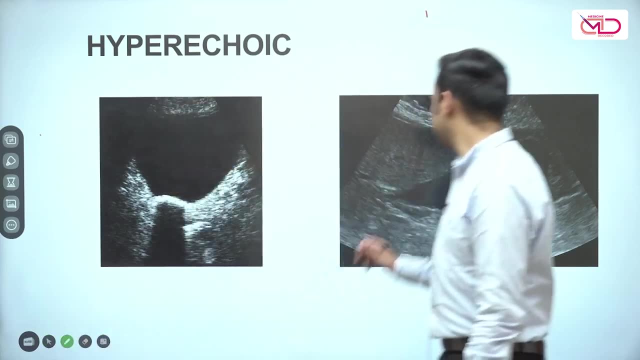 So let us look at this particular image first, This particular image, as you can obviously see, as I told you in the last section, of anechoic structures. now you can see that this is a structure which is anechoic, It is a pier-shaped structure. 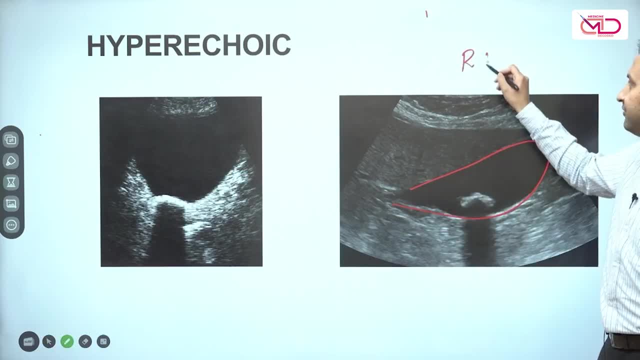 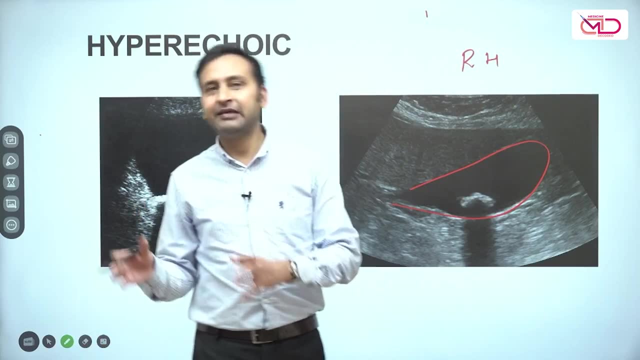 And if I tell you I was imaging right hypochondrium while I was imaging this structure, then obviously anybody can say that this pier-shaped looking structure, which is anechoic, is going to be some form of bladder, And the bladder which is present in right hypochondrium is the gallbladder. 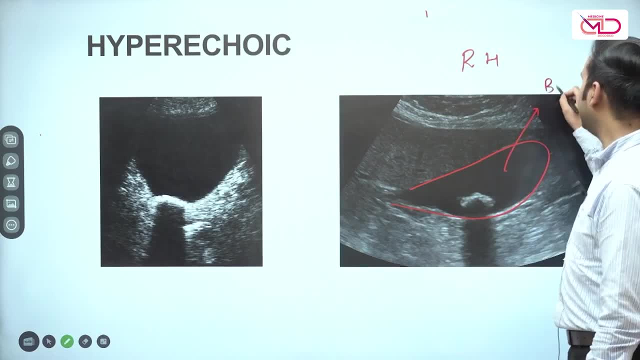 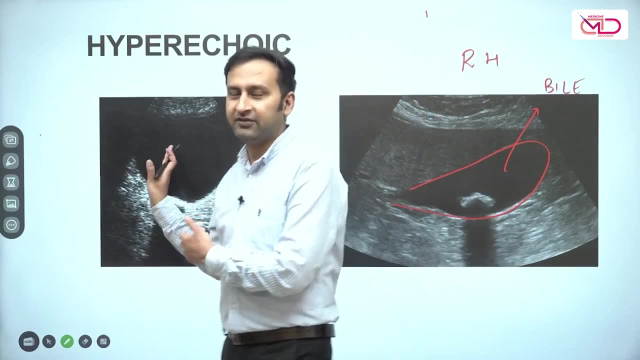 Now, this gallbladder contains fluid. Fluid is bile. Bile is anechoic, So this is going to be definitely anechoic. On the other hand, this particular structure- we just saw in our previous slide that a quadrilateral structure which is present just beneath the skin surface- is nothing. 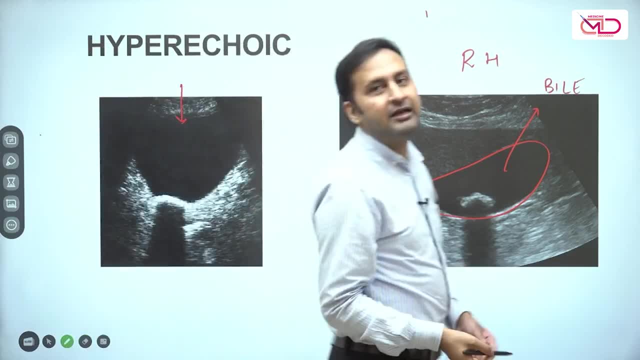 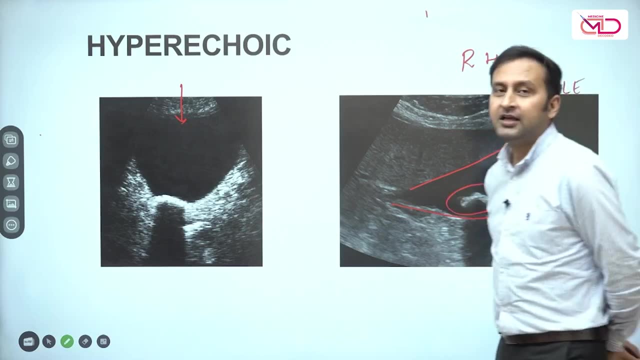 But a urinary bladder which contains fluid, because it contains urine which is completely anechoic. But that is not all. Now you see that there is inside this gallbladder, we can see a structure which is very, very white or very, very bright on sonography. 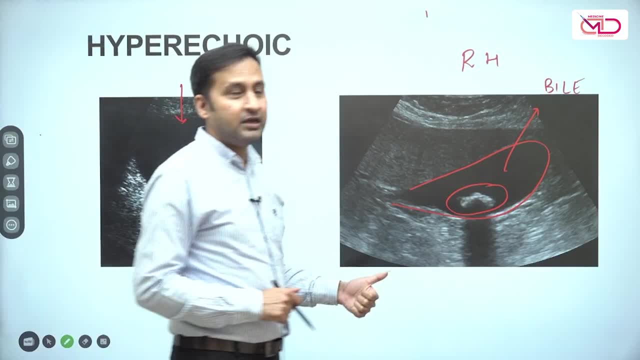 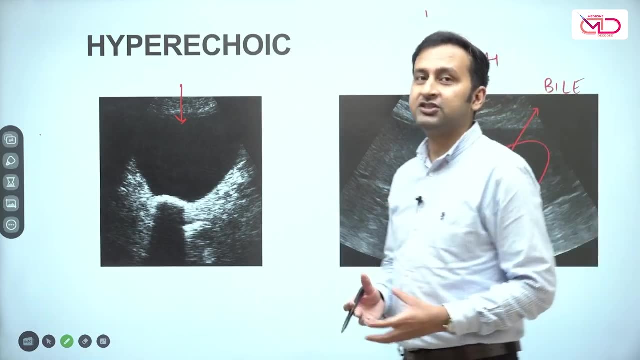 So this structure, which is very white and very bright on sonography, must be a hard structure. So what do you expect? A substance which is very hard, which is present within the gallbladder, which is producing a very bright image. So it has to be a gallbladder stone. 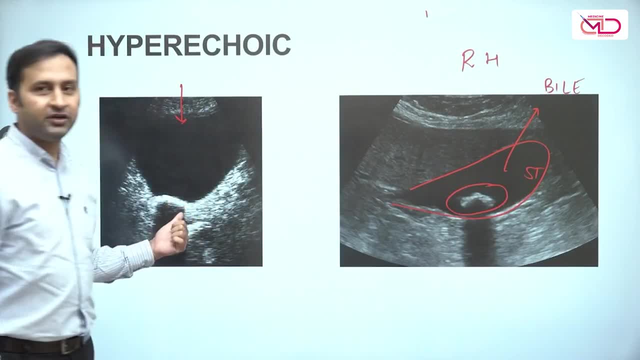 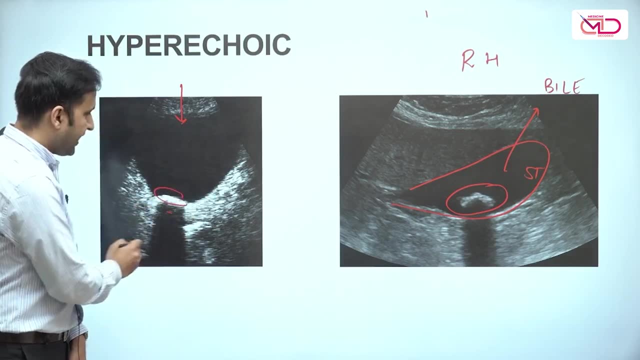 And that is it, Thank you. And similarly, this is a urinary bladder, or you can see, on the dependent wall of the urinary bladder, there is a structure which is white, There is a structure which is white, and this is responsible, producing a very hyper-echogenic. 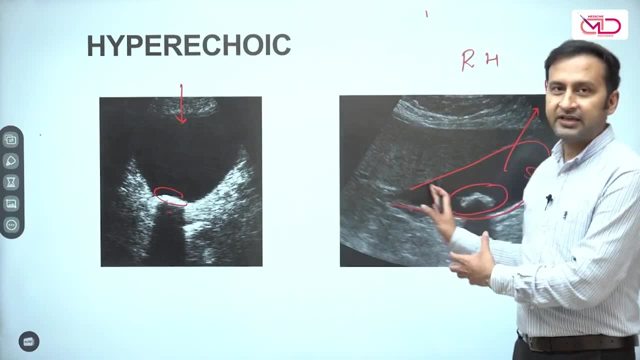 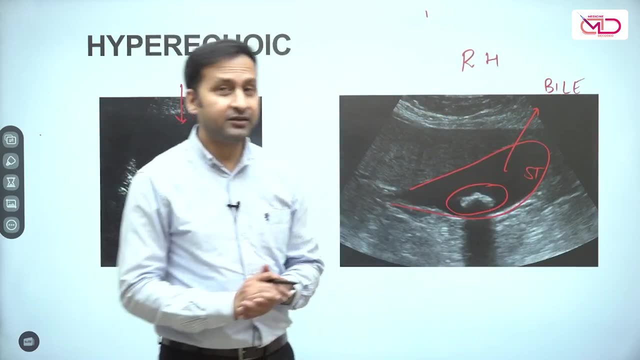 image on sonography. So both of these are stones. One was there in the gallbladder, the other was there in the urinary bladder. Now, one more thing which you all also need to see is that just beneath this particular stone is a black colored shadow which is there. 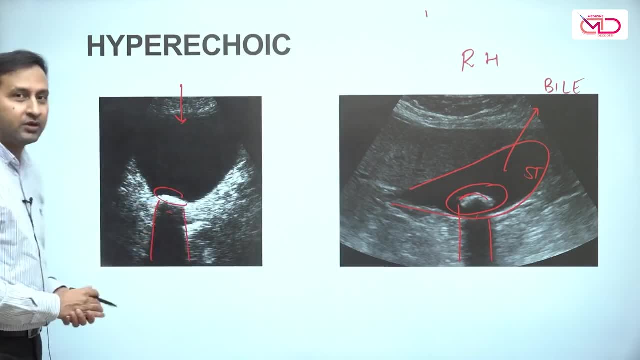 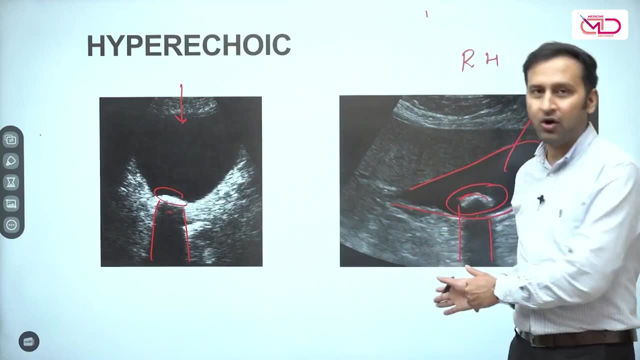 You can see that there is a black colored shadow which is produced by the stone. Now why this shadow is being produced? It is being produced because it is a very strong structure. It doesn't allow any sound waves to pass beyond it. All the sound waves are reflected and, as a result, we cannot image anything beyond it. 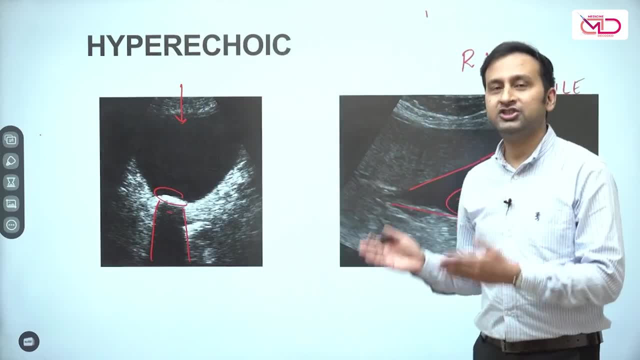 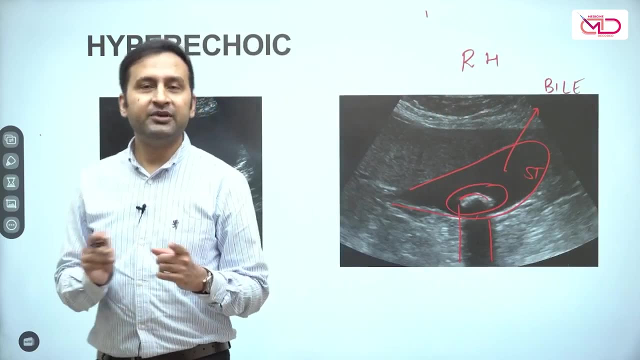 In our terminology of radiology we call it as acoustic shadowing, and it is very classical for all calcified substances like stones, as well as bones, And this is the reason why, for imaging bones, ultrasound is not the imaging modality, because our bones will react. 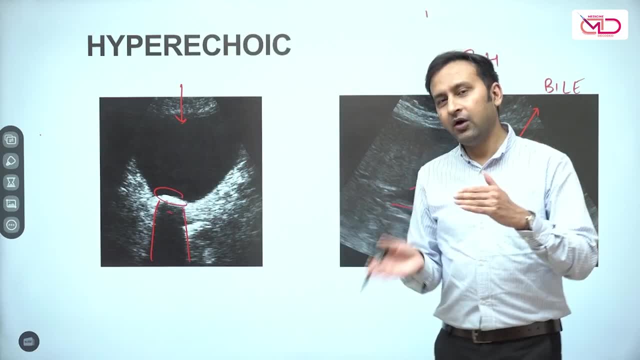 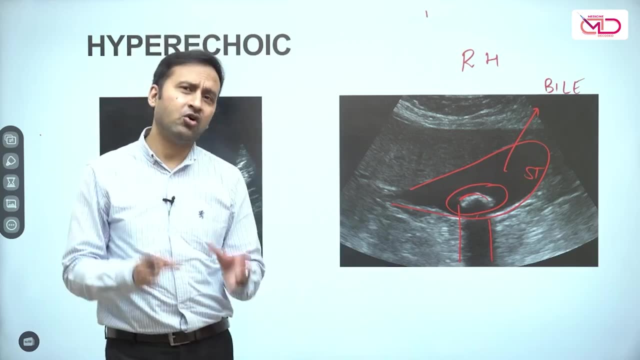 They will reflect almost all the sound waves and they will not allow anything to pass beyond them and, as a result, we cannot see or visualize the medullary cavity of the bone, which is the seat of most of the infections or the malignant or any other processes in the body. 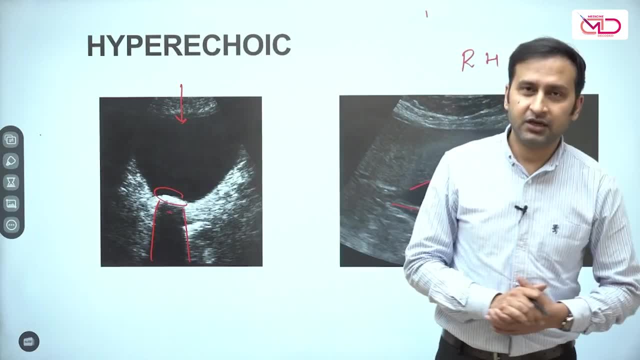 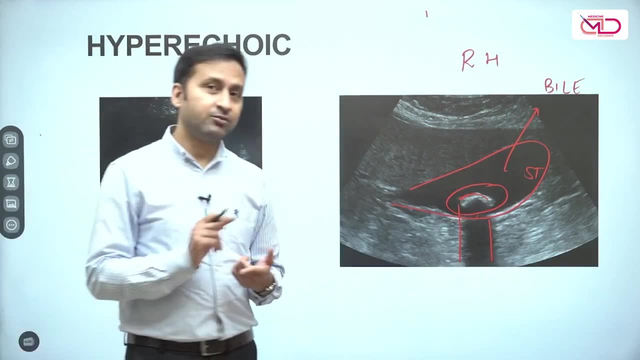 And inside that, there is one more addition I would like to make. when we are discussing about the anechoic substances, We have discussed about the bladder, we have discussed about cysts, we have discussed about cavities, but we haven't discussed about fluid, which is there at one more place in our body. 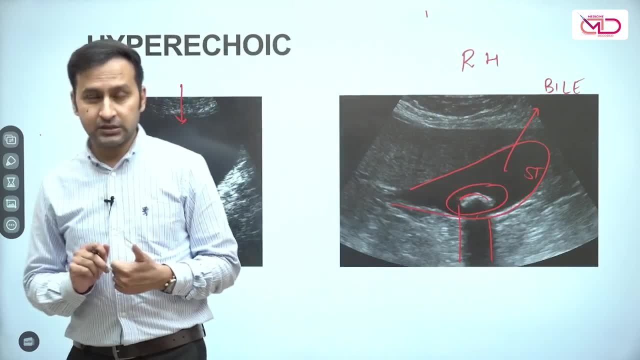 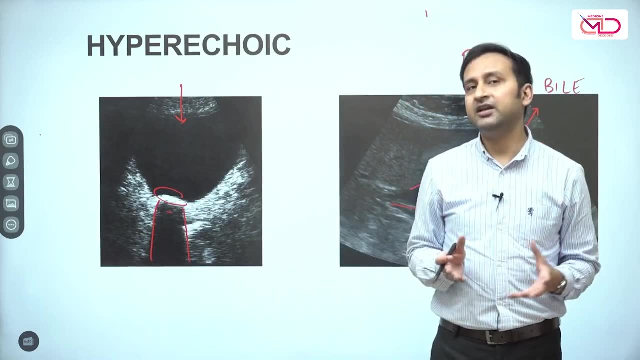 which can be imaged by sonography And that is in the blood vessels. The blood within the blood vessels, the fluid is moving, Similarly as in the heart. heart also contains fluid, So it can be very well imaged on sonography and it will appear anechoic. 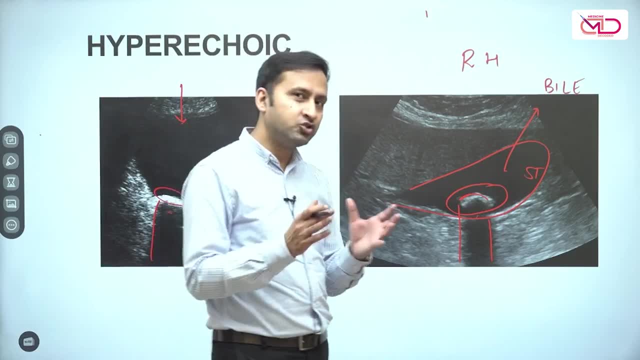 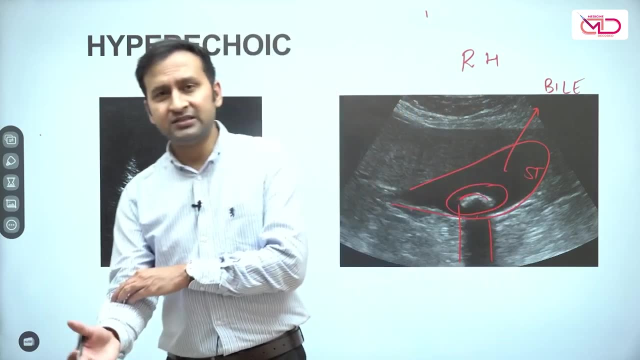 And anywhere. when you see a linear, anechoic structure in the body, it has to be some form of a tube, and any of the tubes which are present in the body which transmit fluid are only blood vessels. They could be veins, they could be lymphatics or they could be plane arteries. 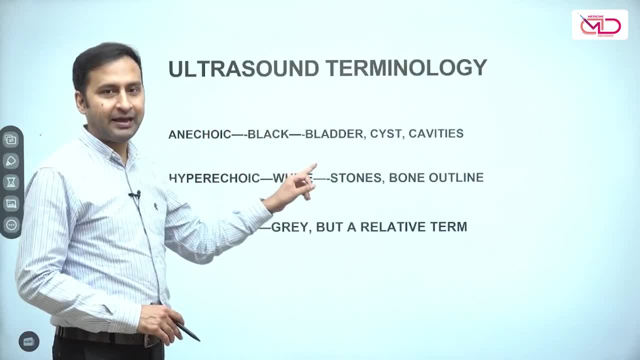 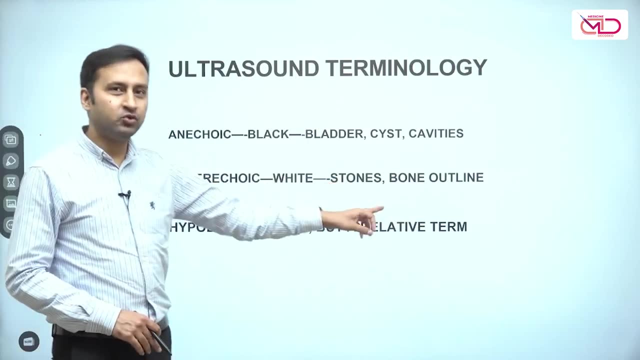 So revising the basics again. Anechoic, no echoes. black bladder cysts, cavities are going to be looking black. anechoic, Hyperechoic are white. All the stones and the bones are going to appear bright on its own. 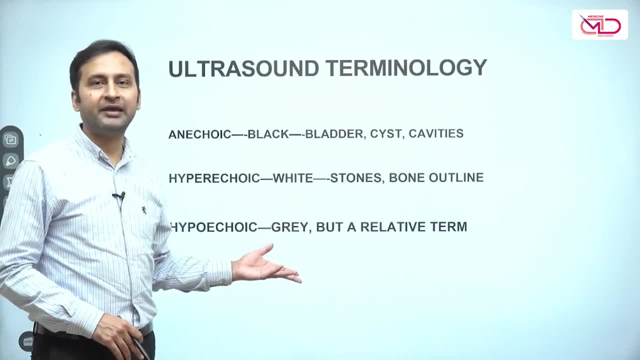 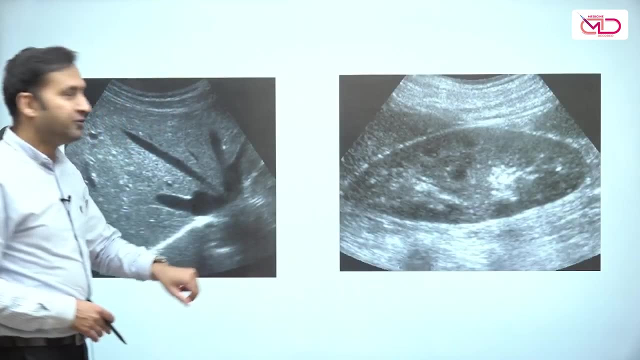 And hypoechoic is a related term. These substances are going to appear gray. They include all solid organs like kidneys and liver and pancreas and all and so on. So when you talked about the gray colored or the hypoechoic or isoechoic thing, I need 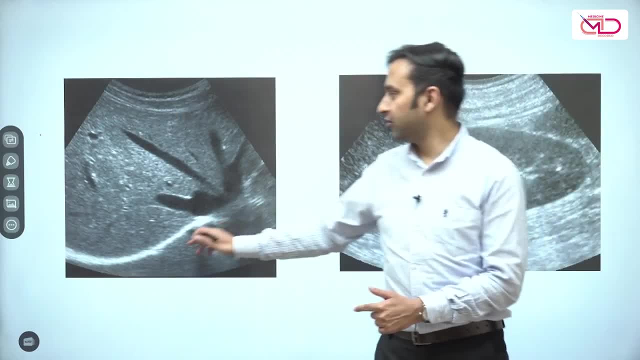 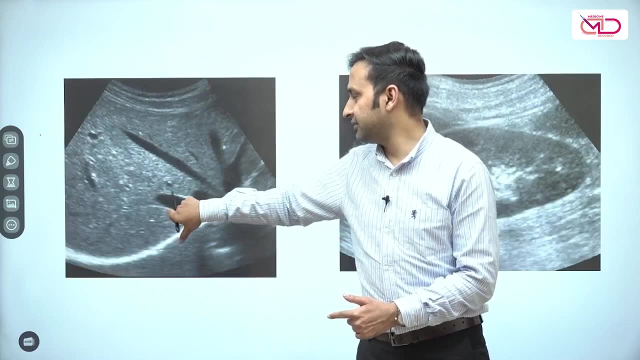 to show two more images to you. This is the one. This is a solid organ, as we can see this because this is not containing any anechoic structures. apart from these three linear anechoic structures, as you can see here, This is the structure which is present in right hypochondrium, the largest organ of 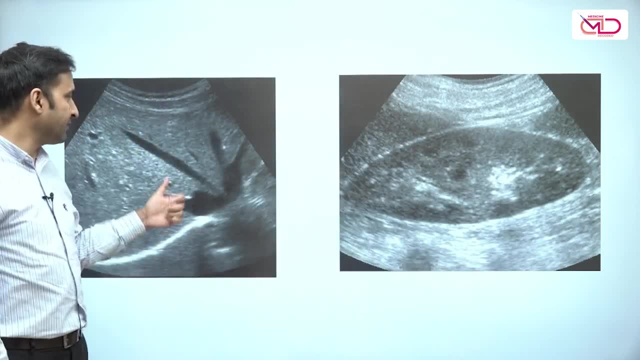 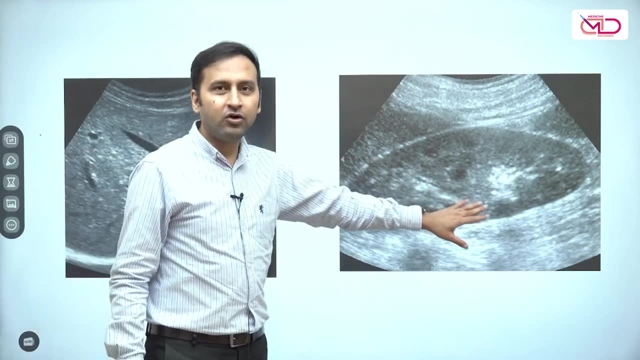 the body. This is liver. largest abdominal organ of the body. this is liver And all what we can see moving around in a linear fashion, which are anechoic. these are the blood vessels. These are the hepatic veins. Similarly, I think all of you can guess, by the shape of this organ. 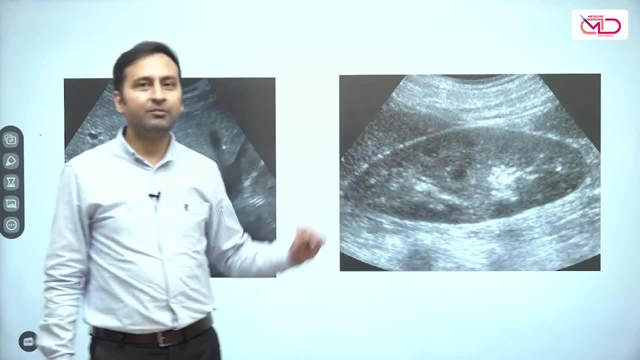 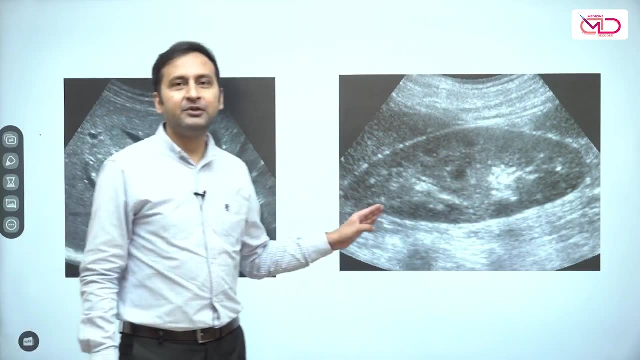 This is not white, so it is not bony. This is not black, so it doesn't contain any fluid or cysts. This is giving a rainiform contour and this is present in lumbar region. There can be nothing else, but this is the kidney. 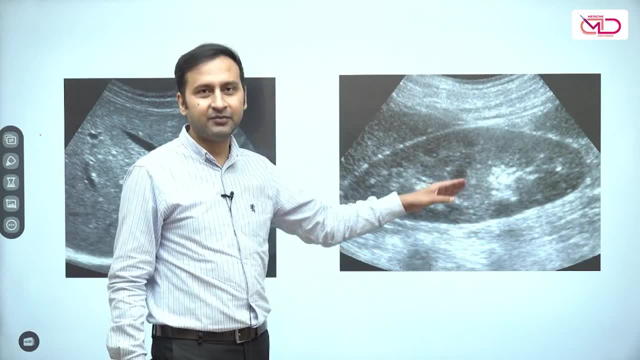 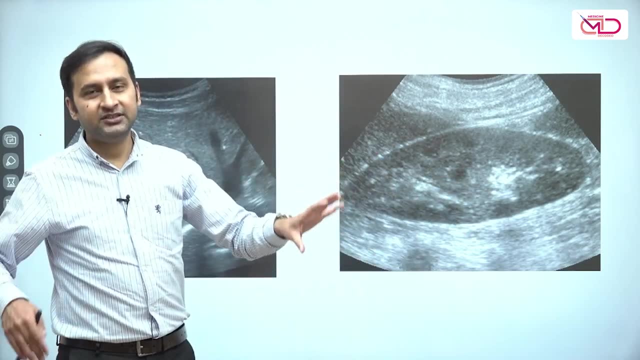 I am not talking, I won't be telling why some things are looking white and some things are looking gray, but this is for a general understanding, for general information. A rainiform shape should give you an indication, while imaging in the lumbar region nothing. 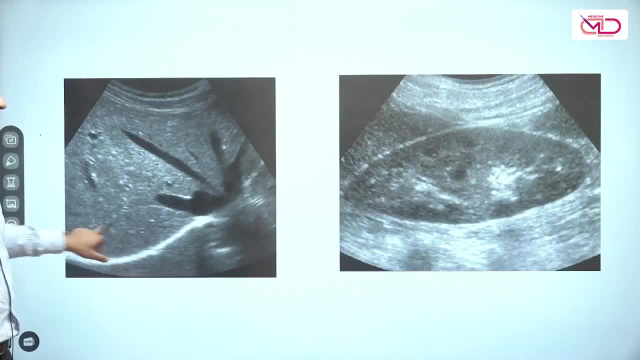 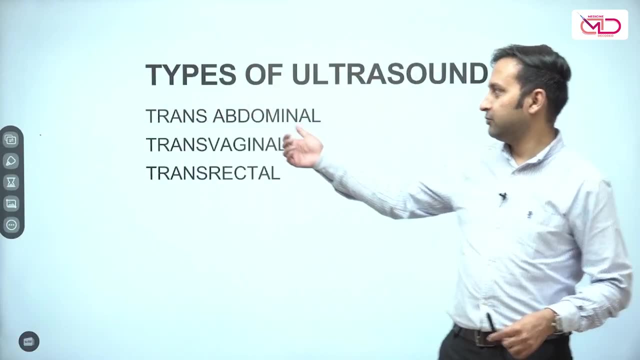 else can be present other than the kidney. So now, coming on to last section of this lecture, which will be focusing on how do we do a sonography. One is the most commonly used is the transabdominal scan, In which the probe is placed over the abdomen. the other is trans-fusional, the others are: 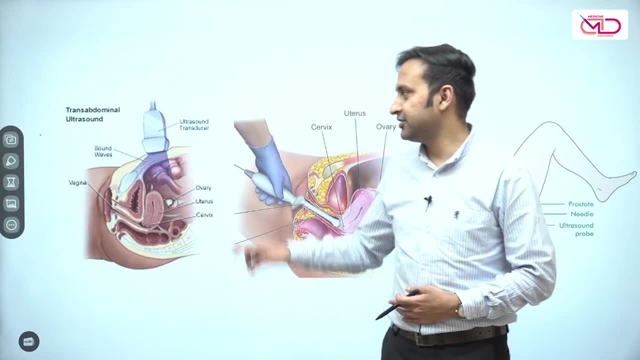 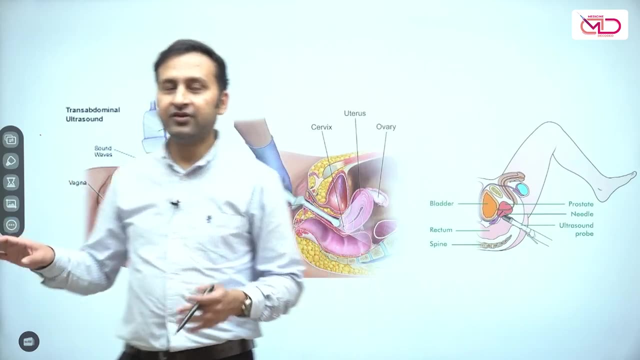 trans-fusional and trans-rectal. These are the endochemistry ultrasound. they are specialized ultrasounds. So this is a transabdominal scan in which the probe is placed over the abdomen for scanning elsewhere. But when we are trying to scan the uterus or we want to scan prostate in males, we should. 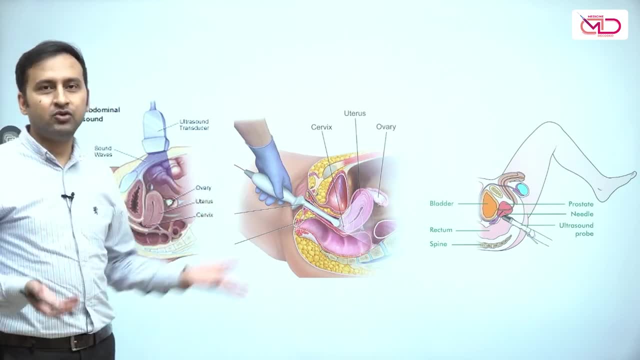 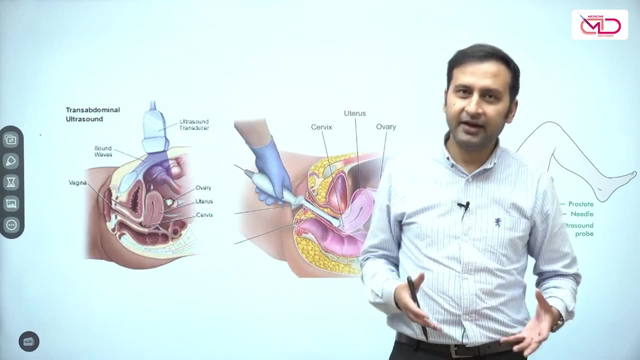 have the bladder full in this particular case. Otherwise, when bladder is going to be empty, first of all bladder itself is not going to be seen and apart from that, the other structures are going to take place of bladder and the optimum utilization of all the pelvic organs in a normal anatomical state won't be possible. 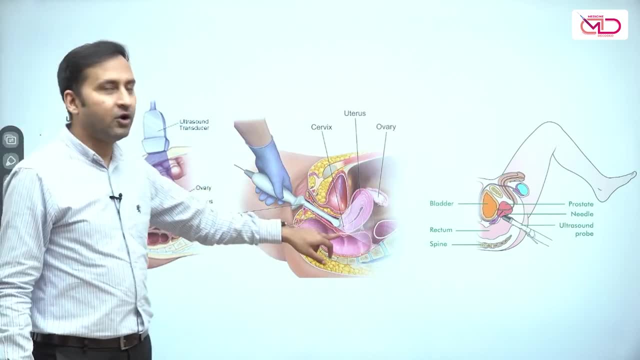 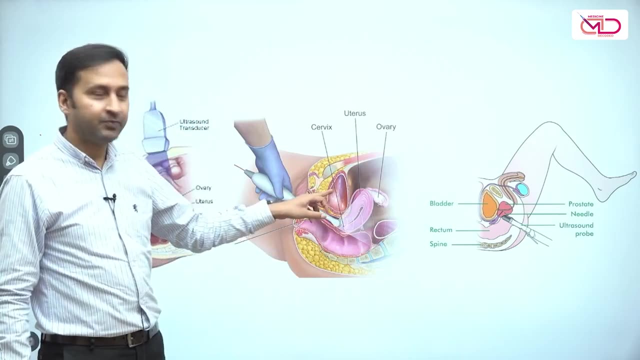 While using a transvaginal probe, the probe is inserted deep down the vagina. So, as you can see that this probe is inserting to the vagina, we almost bypass this: the role of the urinary bladder. Now, as I told you that, when we are forming an image on a sonographic screen, the image 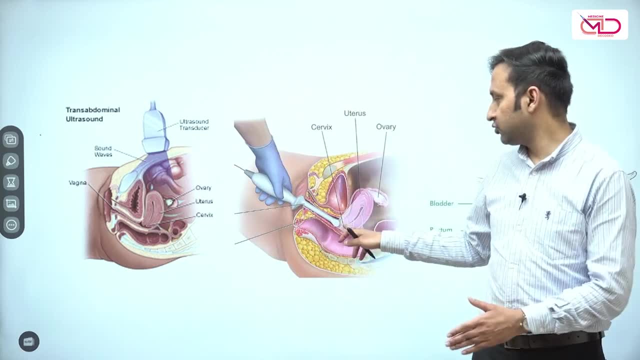 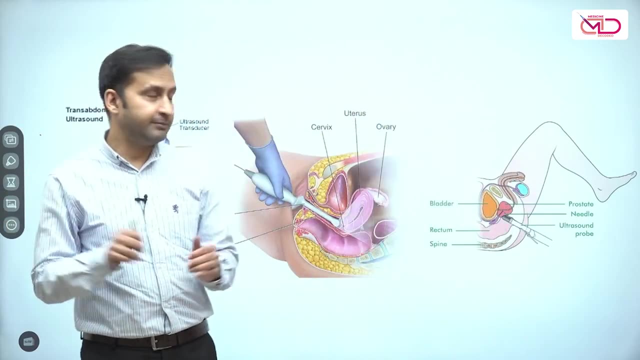 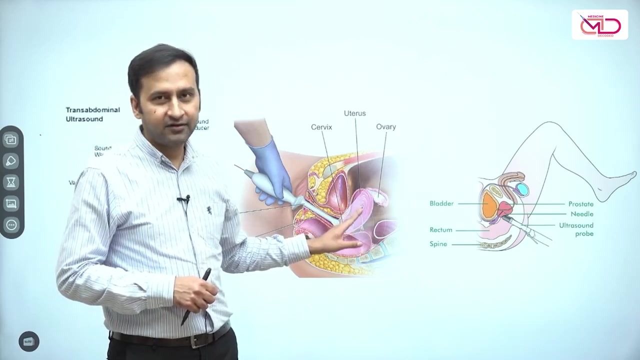 which is closest, the part which is closest to the transducer will form the image first, on the ultrasound or the transducer. So the first image that will be formed in a transvaginal scan is that of cervix. We won't be able to find any bladder in the transvaginal scan because the bladder is already. 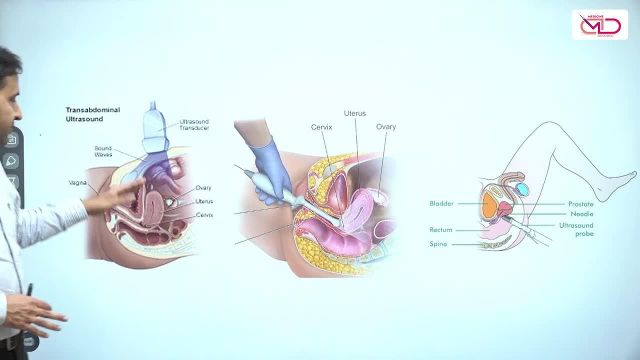 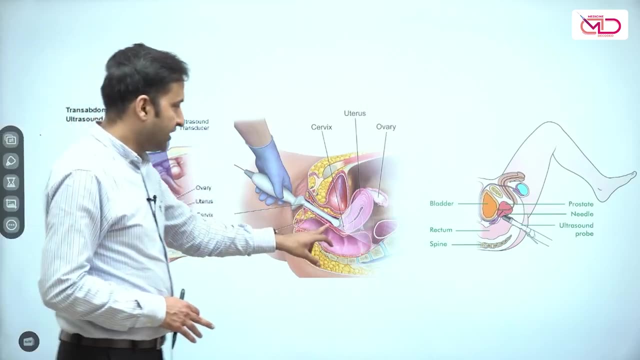 emptied and it is bypassed. Secondly, this image- see the uterus is far behind. So the image of uterus in this particular case will not be much magnified, while a transvaginal scan is scanning only the uterus. So we'll have a much brighter and much- sorry, not much magnified image of uterus on the. 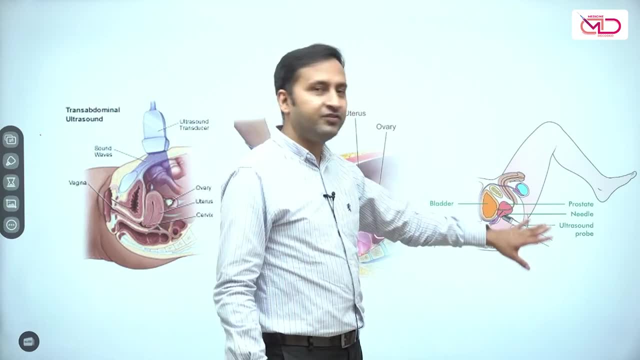 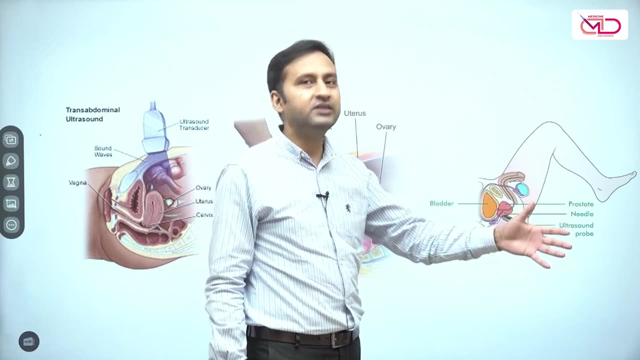 screen while using a transvaginal scan. Transrectal sonography is specifically limited for prostate and it is used to see some prostatic conduce, but it is in clinical practice. its role is significantly limited, Apart from doing biopsies, we usually do not do it on a routine basis. 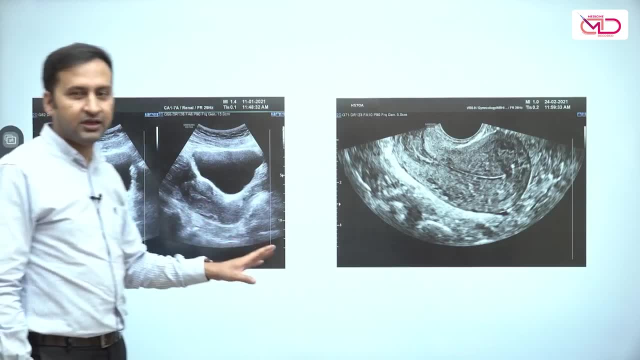 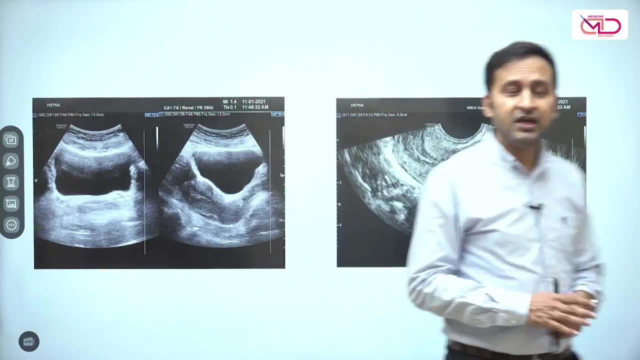 So this: these are the two images of the same patient versus the transabdominal scan. This is important because sometimes you might be given some pictures and patients and you might be asked whether it's a transabdominal or it's a transvaginal sonography. 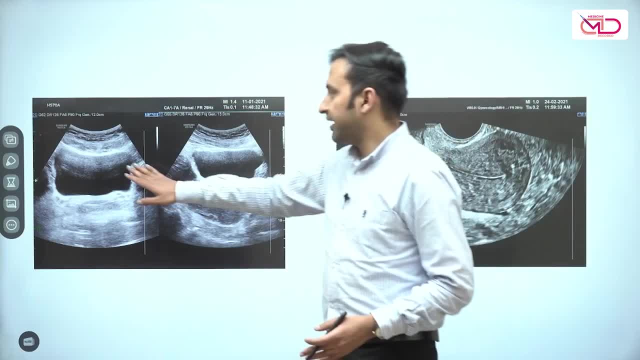 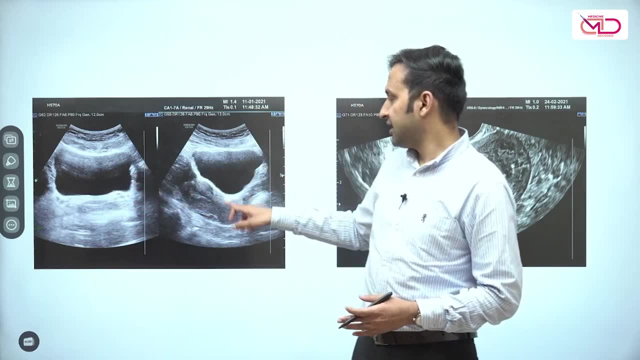 So you can see that there are clear cut differentiating points For transabdominal sonography. the first thing that we see is the bladder, because it is just close. it is the closest to the skin and the subcutaneous veins and behind the 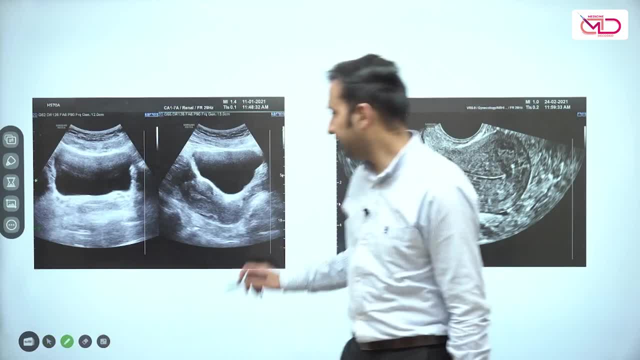 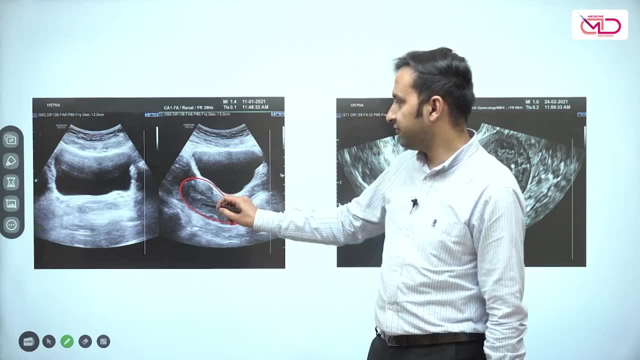 bladder. I'll tell you this is a female patient. So behind the bladder you can see that there is an oblong structure which is present, and this oblong structure is of some grayish color. So it is a structure which is a solid structure. 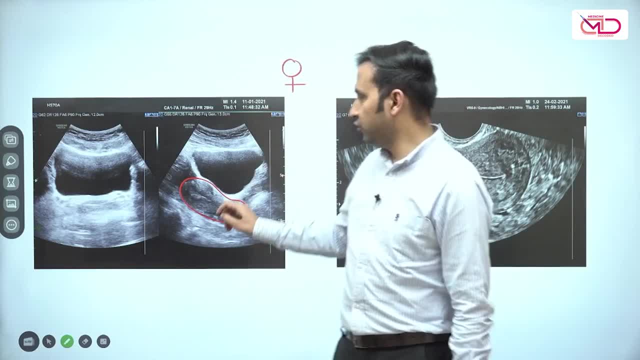 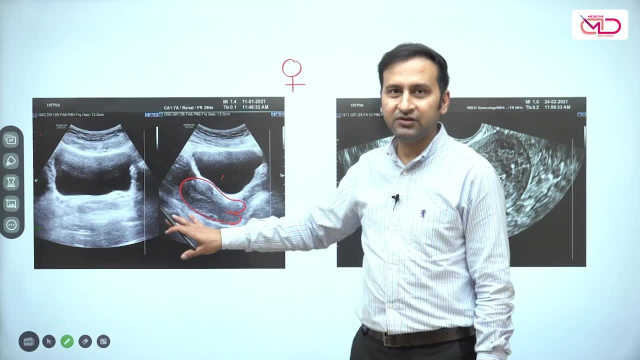 This is a female patient. anything which is present behind the uterus, behind the bladder, which is oblong in shape, This is the uterus, But when we look at it, we can clearly see that the image is not very clear. We can see that there is a bright central line, but we cannot clearly distinguish its. 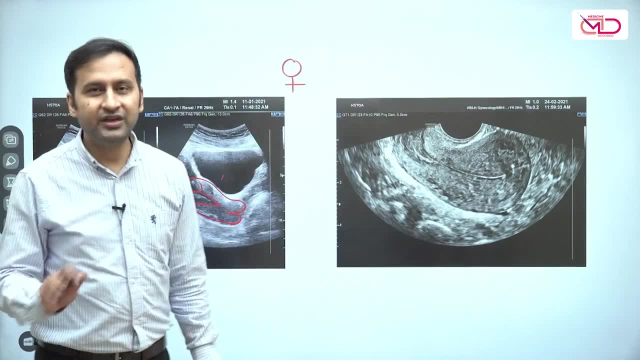 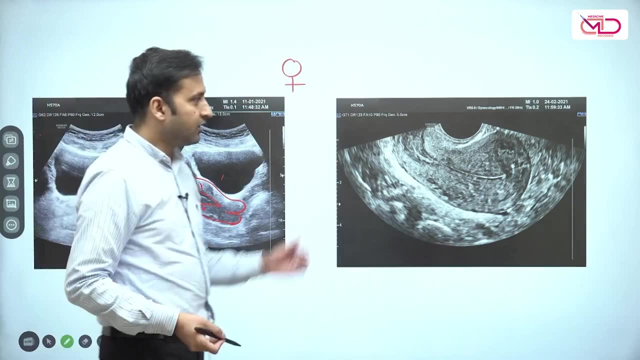 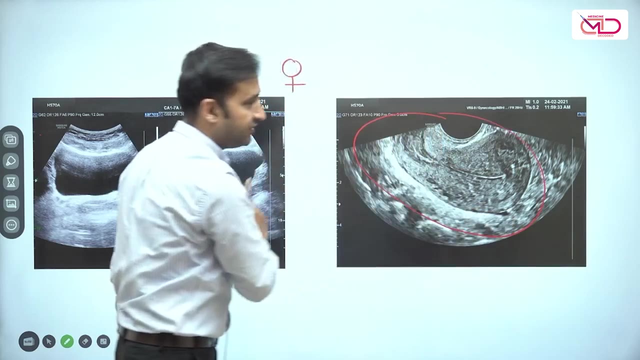 margins and obviously we cannot even see the uterine walls very clearly. Like a very small soft tissue tumor here or there, or myoma may easily be missed. on this scan Now, compared with this scan- this is again of the same patient- See that the image of the uterus is far more magnified in this particular case. 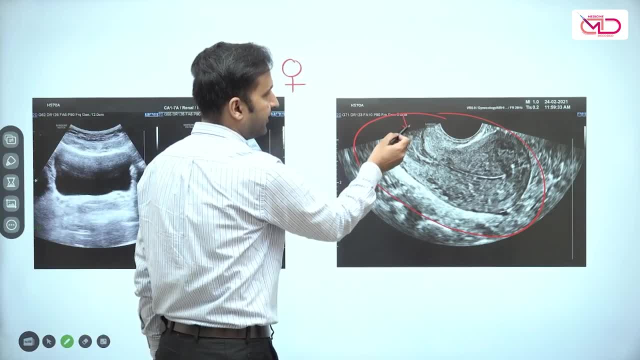 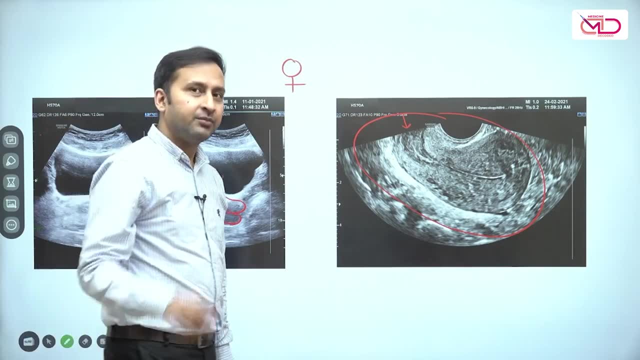 Firstly. Secondly, The only image is the uterine cervix or the uterus directly. We have bypassed the bladder. There was no use of bladder. There is no image of bladder on a transvaginal scan Because? firstly, because obviously the transducer touches the cervix first. 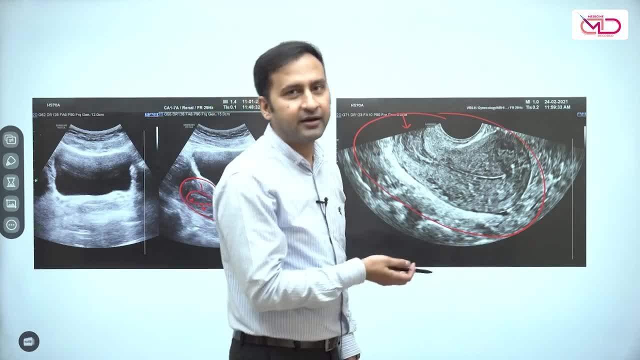 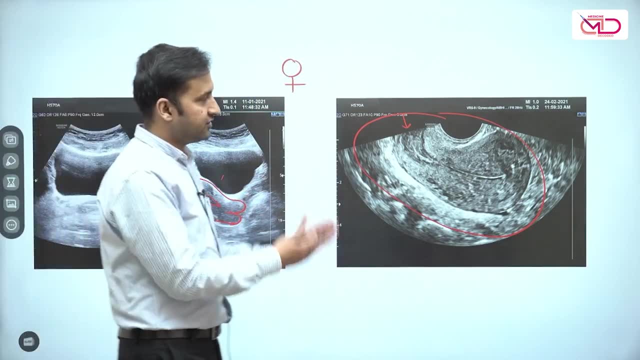 Secondly, because we have emptied the bladder. We do not need to see bladder in this case. So these are two or three major differentiating points between a transabdominal and transvaginal scan. Looking at the transvaginal scan of the uterus or more closely you can see uterus is a classical 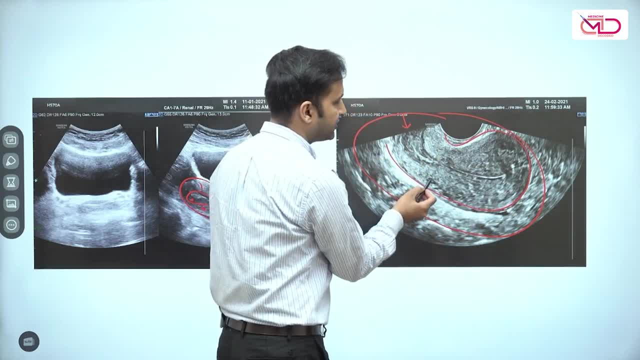 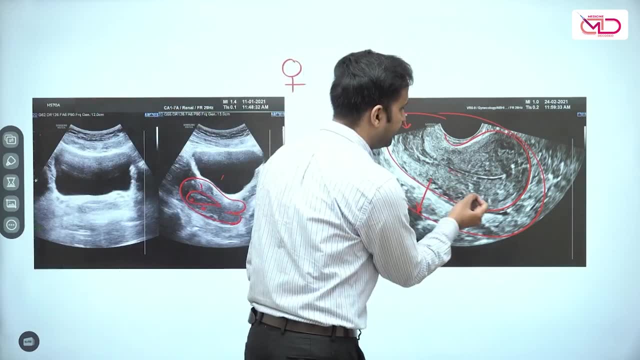 globular organ. This globular organ is used. It is good. It is something which is gray colored because it is a soft tissue organ. It is not a cystic organ. Secondly, we can see that there is an inner lining which is giving us some color. 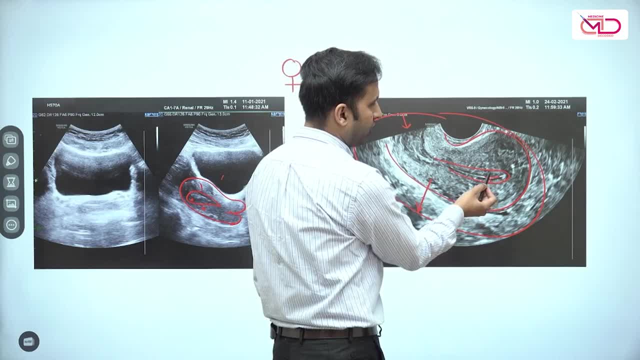 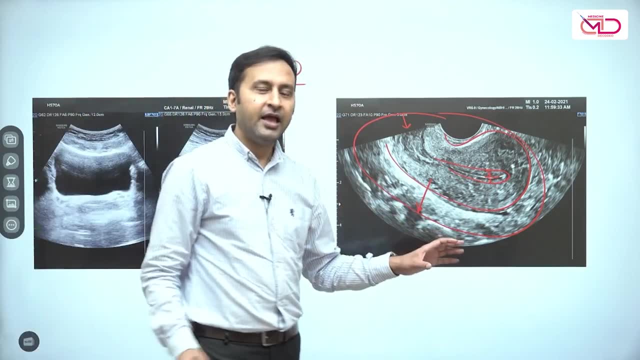 The central part is bright. The outer part is somewhat gray or brown or hypoechoic, you can say The central part is echogenic. This is the endometrial cavity. Endometrial cavity behaves this way and it changes its size, It changes even sonographic morphology in different phases of menstrual cycle, which 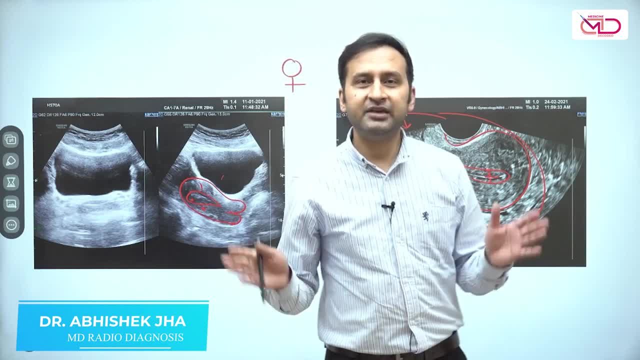 we will be discussing in our subsequent sections. So this was a basic lecture about how do we see and how does an image form on a sonography.